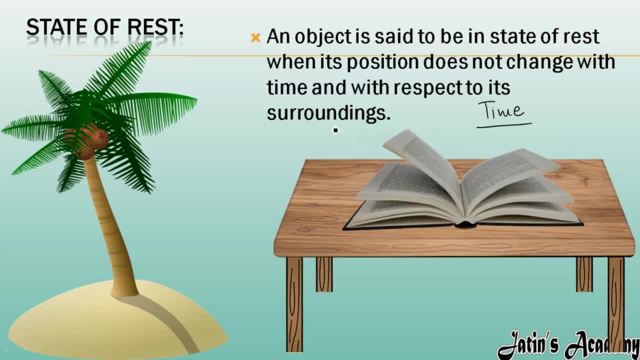 its position with respect to time plus with respect to surrounding. also, Book is on same place, So you can say that book is in the state of rest. Similarly, you can see this table also. This table is also not changing its position. This table is on same position. 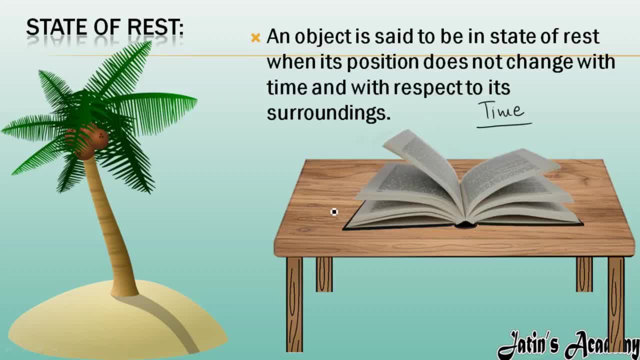 no, So table is also not changing its position with respect to time, with respect to surrounding, So this table is also in a state of rest. Then we are having this example of tree. This tree is also on the same position, same position of ground. 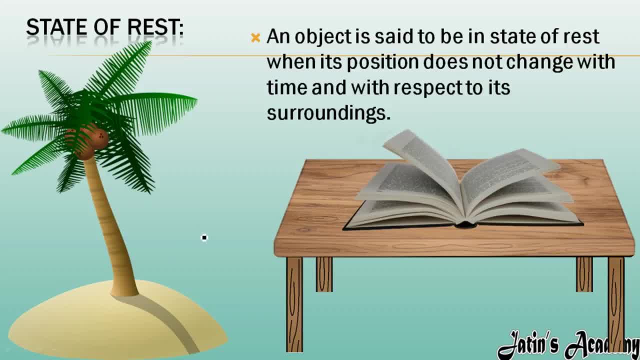 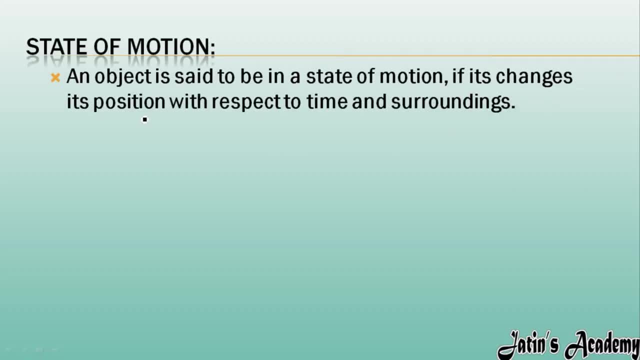 So that tree is also in a state of rest. So next we are having definition of state of motion. So what do you mean by state of motion? An object is said to be in state of motion if it changes its position with respect to time and surrounding. 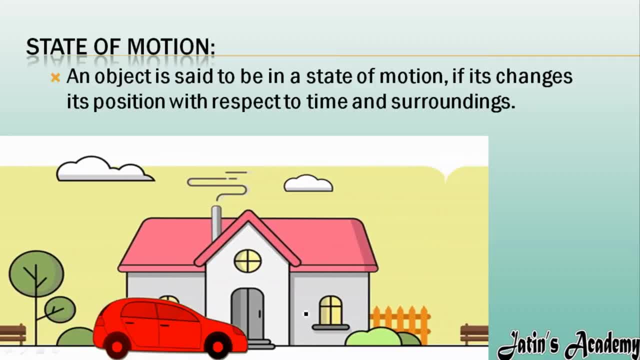 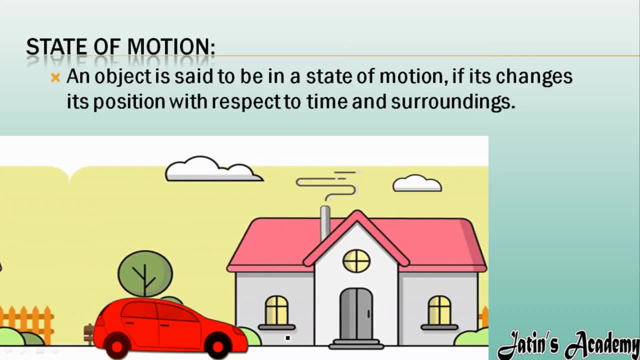 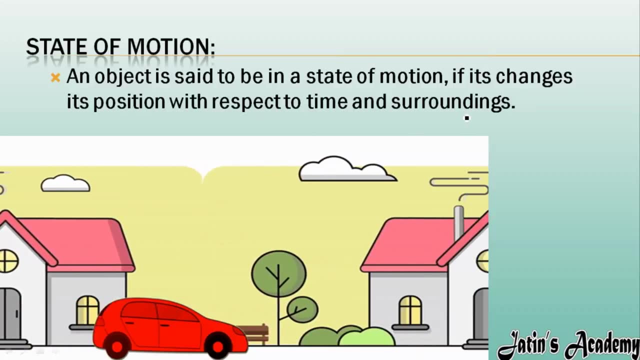 How, For example, this car is moving. So this car is changing its position. Firstly, this is on this place, Then afterwards it go near to house, Afterwards it go near to this trees and all. So this car is changing its position with respect to time, with respect to surrounding. 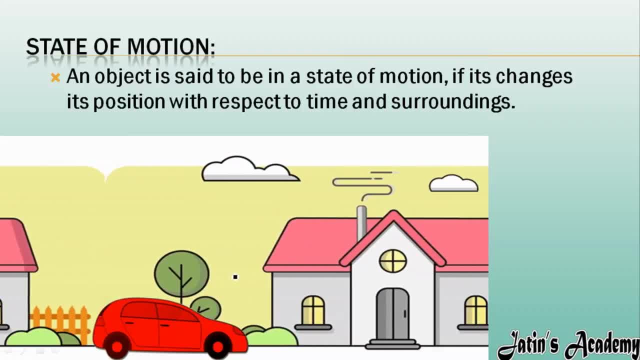 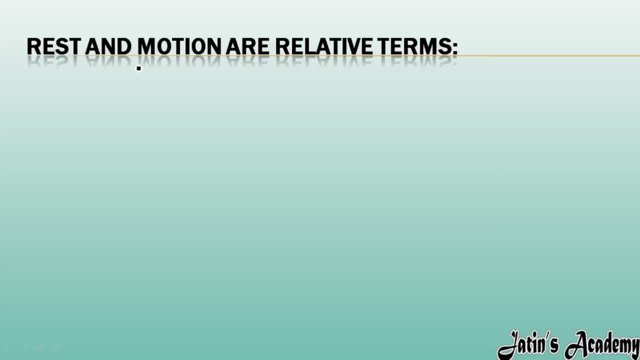 So whenever any object changes its position, that object is said to be in a state of motion. Fine, So next we are having rest. Rest and motion are relative terms. What do you mean by relative terms? Relative term means rest and motion. they both are dependent on each other. 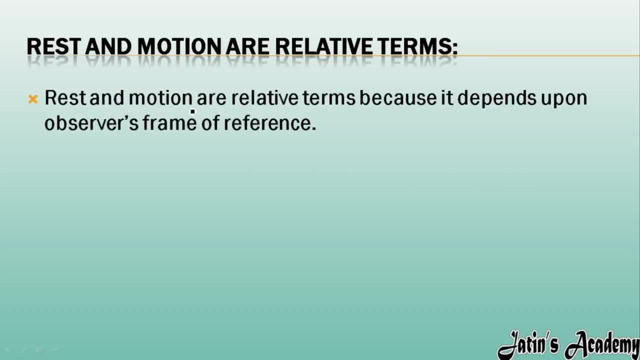 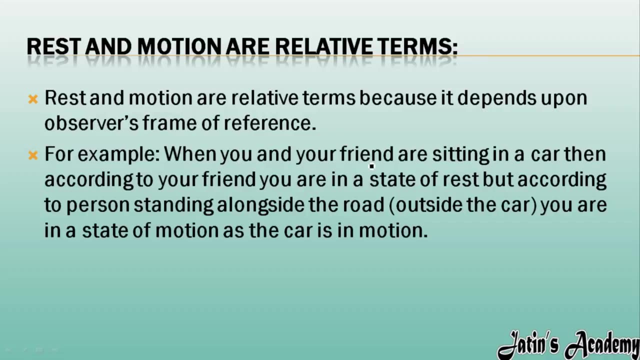 How dependent on each other. See carefully. Rest and motion are relative terms because it depends upon observer's frame of reference. How it depends upon observer's frame of reference, See by taking an example. For example, you and your friend, you both, are sitting in a car. 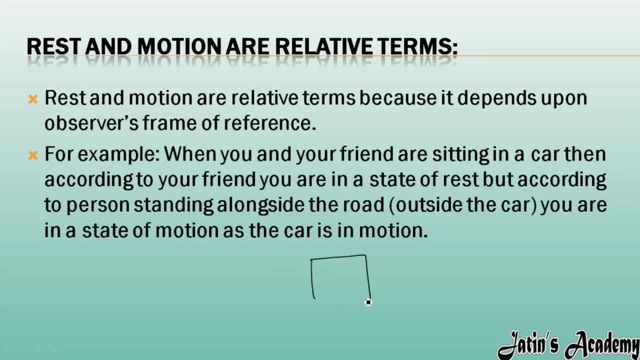 Okay, For example, you and your friend. for example, this is a car, you and your friend, you both are sitting in a car. Fine, Then, according to your friend, this is you. this is your friend. According to your friend, you are in a state of rest because in car, you are not moving here and there. 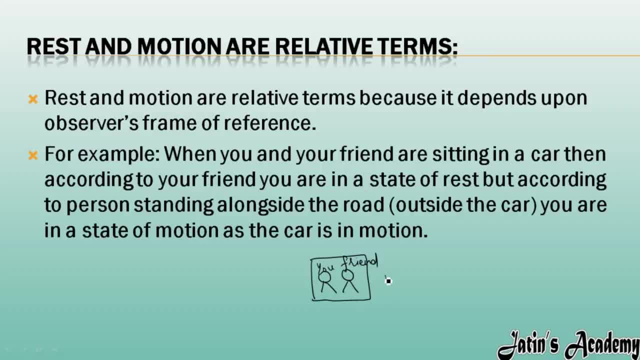 You in car, you are sitting on one place, Fine, But your car is moving and the person who is standing outside the car, That person, what he will say? he will say that now you are in motion because, according to this person, you are changing your position with respect to time, with respect to surrounding. 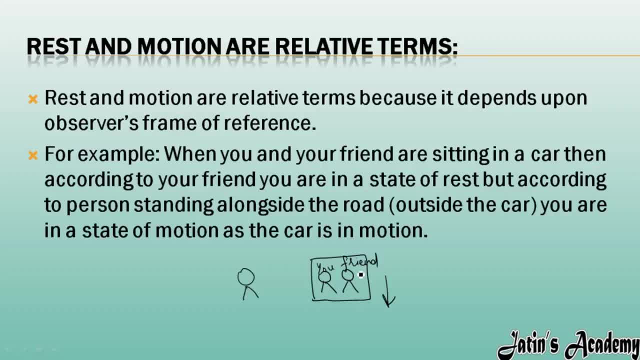 So according to this person, you are in motion, But according to your friend, which is sitting near to you, according to your friend, you are in a state of rest. So it all depends upon observer's frame of reference, that what observer is watching. 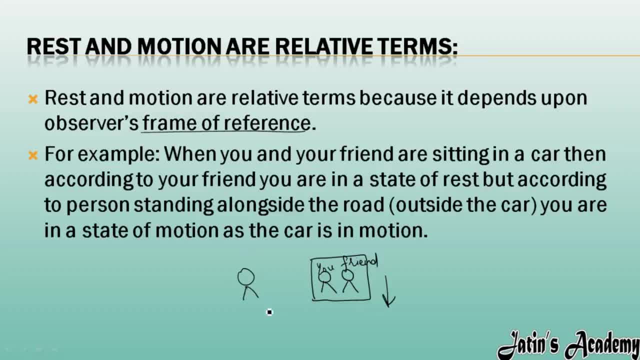 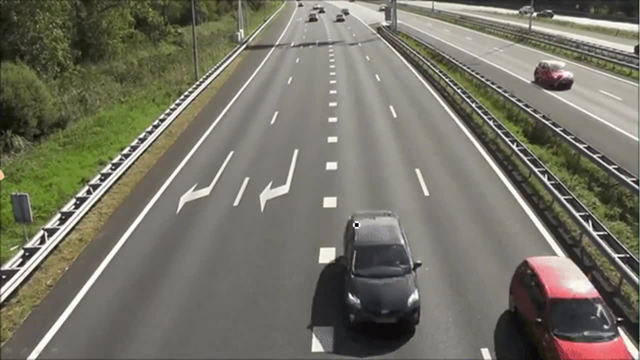 That? what observer is thinking? So, according to this observer, you are in a motion, But according to this observer, you are in a state of rest. So state of rest and motion, they both are relative terms. See, for example, this is a car in which you are sitting. 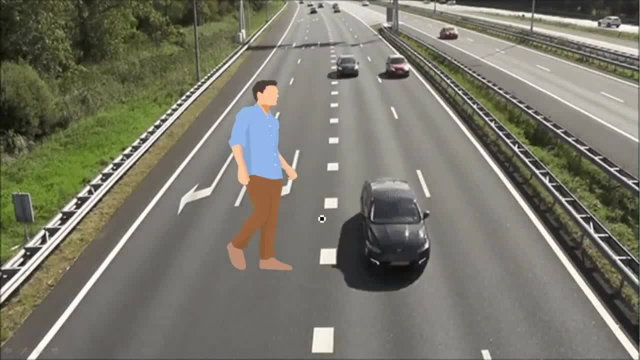 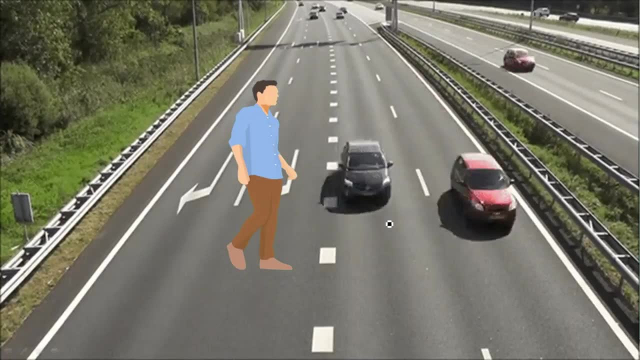 Then afterwards, one boy is standing near to your car. So, according to this boy, you are in a state of motion, but whatsoever, your friend is sitting inside the car. Okay, According to that friend, you are in a state of rest. 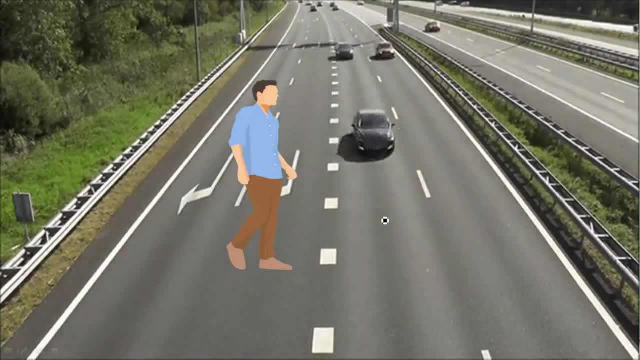 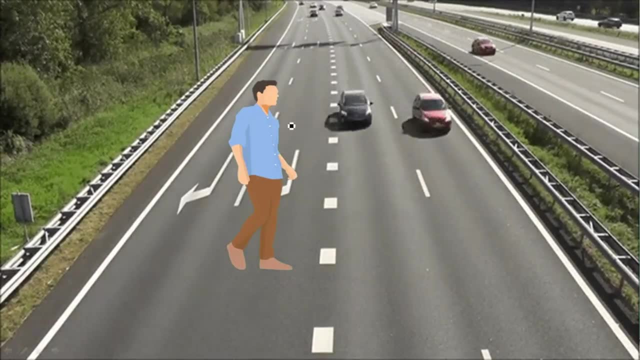 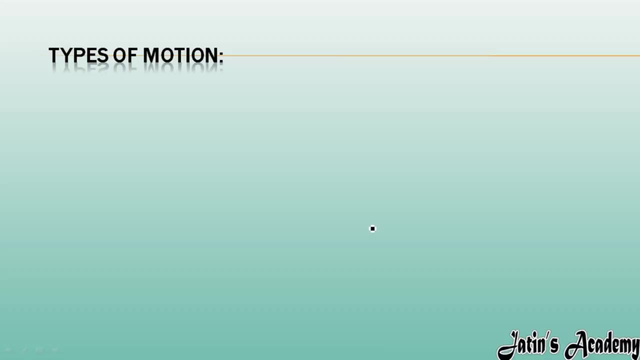 So rest and motion, they both are relative terms. Relative term means they both depend upon observer's frame of reference. So here two observers are there: One observer is standing outside your car and one observer is sitting with you inside your car. Next topic we are having here: types of motion. 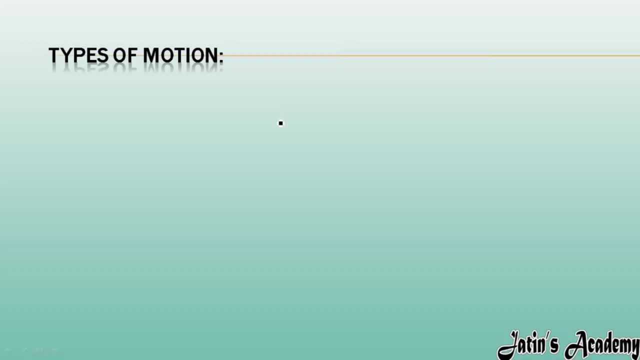 So here in this chapter we are going to learn about the different types of motion. So their name is: translatory motion, rotatory motion, oscillatory motion, multiple or complex motion, periodic motion, non-periodic motion. So here we are going to discuss about these six types of motion. 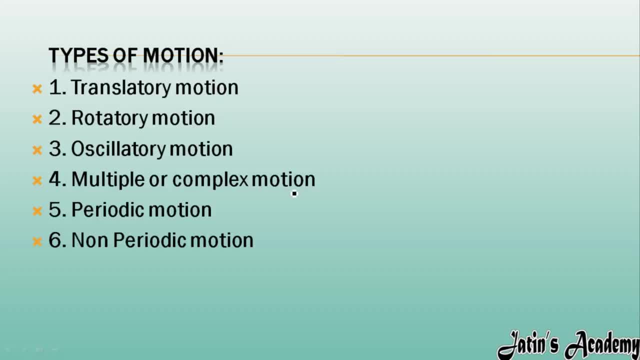 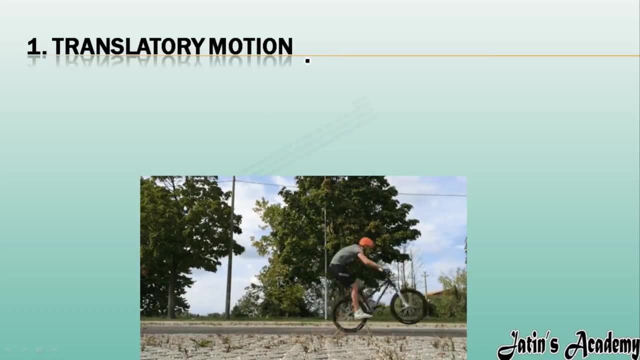 Plus this, we are going to discuss about uniform and non-uniform motion also. Fine. So these motion we are going to discuss, with their definitions, with their appropriate examples also. So First type of motion is translatory motion. So see carefully, what do you mean by translatory motion? 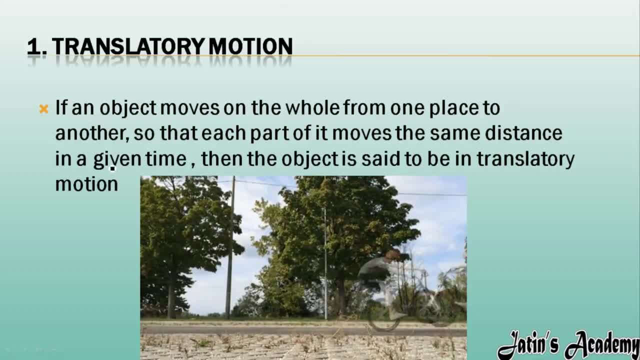 If an object moves on a hole from one place to another. when this object is moving from one place to another, for example, this person is here, This person is changing its position means in five o'clock He's standing here and at five ten. 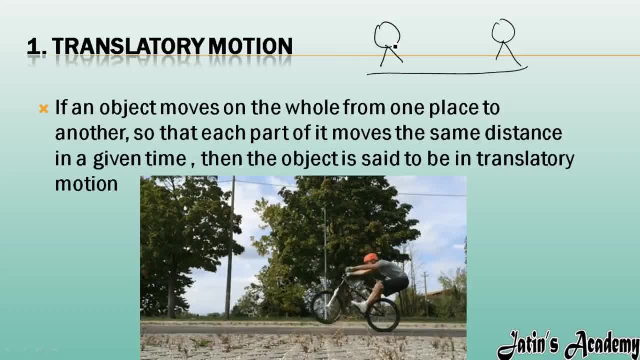 He's standing here, for example. Okay, So when person Moves on a hole, his full body is only moving, So person moves on a hole from one place to another place, So that each part of it moves same distance in a given time. 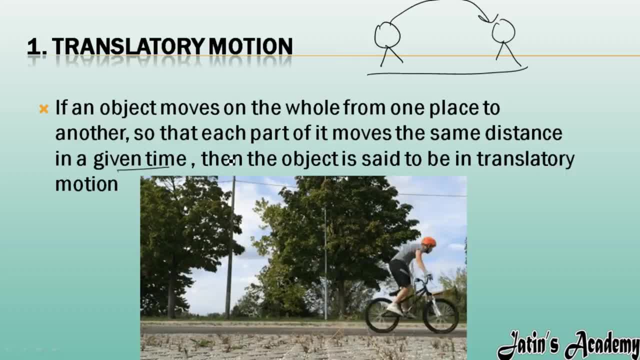 Each part of this body moves the same distance in a given time. So that object is said to be in a translatory motion. See, this bicycle is moving from one place to another. So this whole bicycle is moving from one place to another And it is governing same distance in a given time. 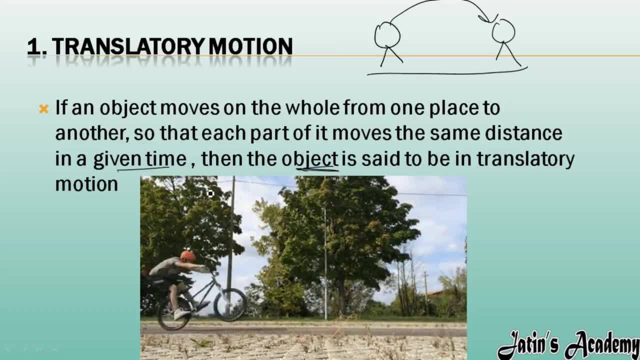 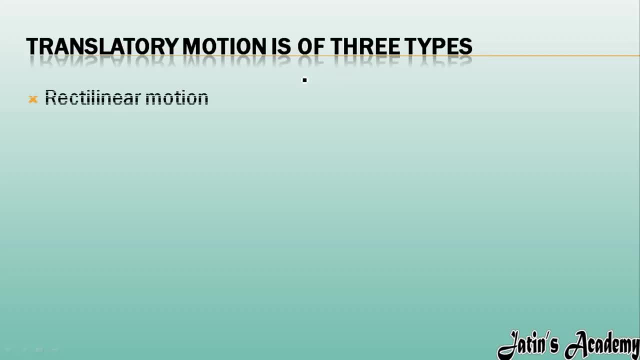 So this bicycle or this boy is said to be in a translatory motion. Next we are having further. translatory motion is of three types. that is rectilinear motion, curvilinear motion. Then we are having circular motion. So here we are going to discuss about these three kinds of motion. 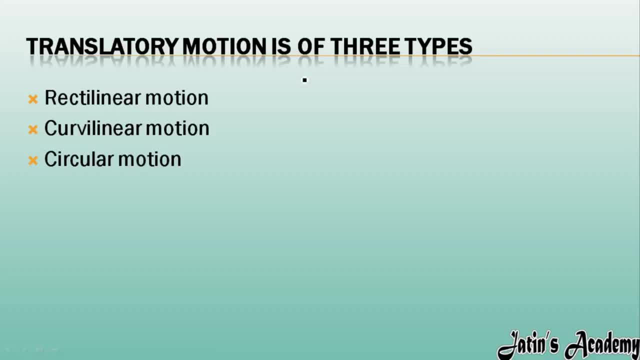 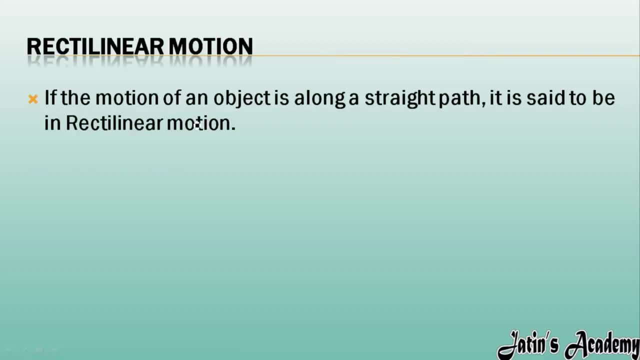 Plus we will discuss what is the main difference between curvilinear and circular motion. So first type of translatory motion we are having that is rectilinear motion. What do you mean by rectilinear motion? If an, if the motion of an object is along a straight path? 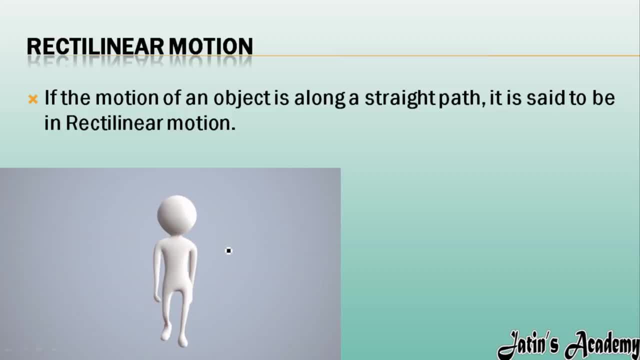 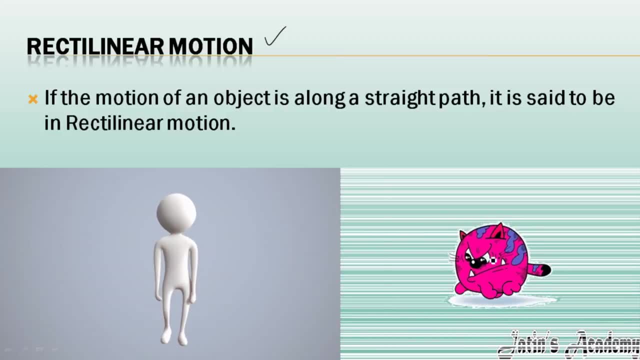 when object is moving in a straight path, then that object means is in which motion it is. in rectilinear motion, See this example. Also, this cat is moving in a straight direction. So when any object is moving along a straight path, so 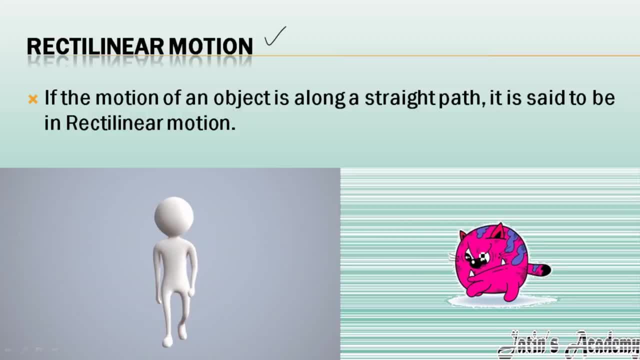 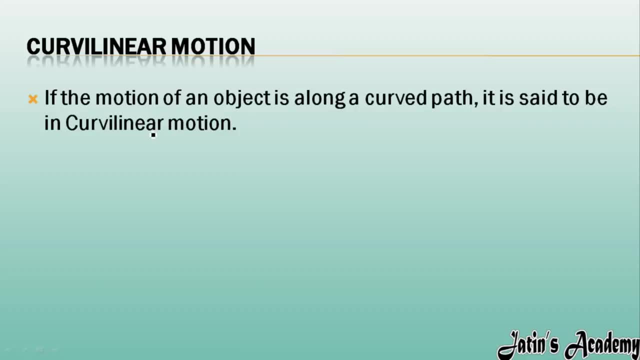 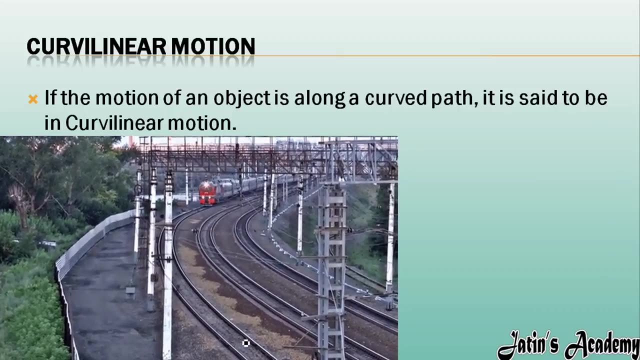 that objects motion. is which motion? Yes, it is rectilinear motion. Next we are having curvilinear motion. What do you mean by curvilinear motion? If the motion of an object is along a curved path? see, this train is going to move in this curved path. 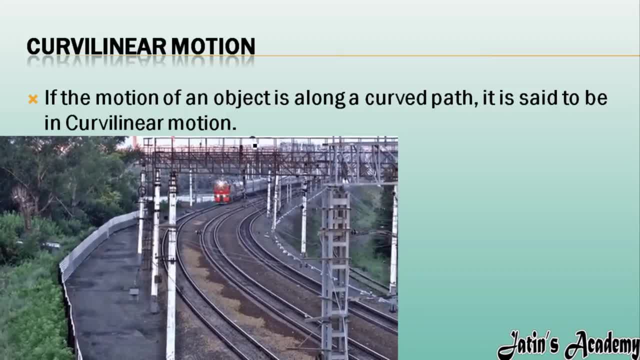 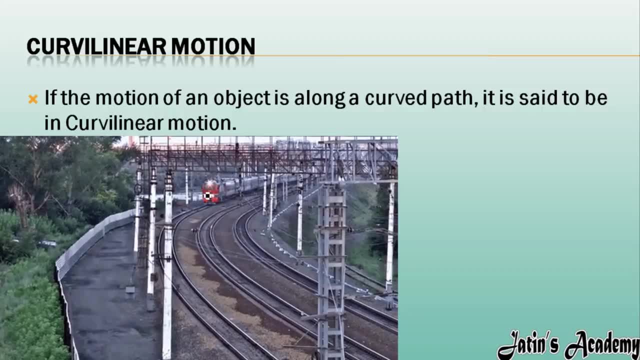 So when object is moving along a curved path, that object is said to be in a state of curvilinear motion. Okay, curvilinear motion means when a motion of an object is along a curved path, that is a curvilinear motion. 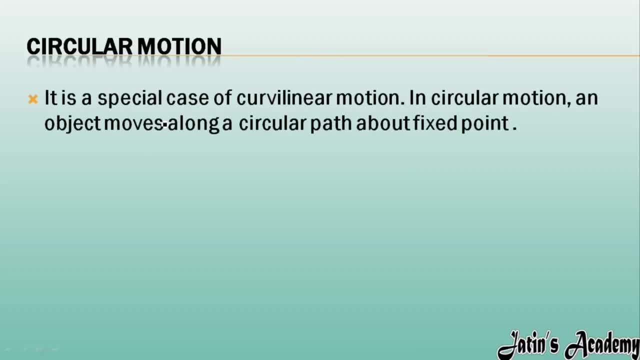 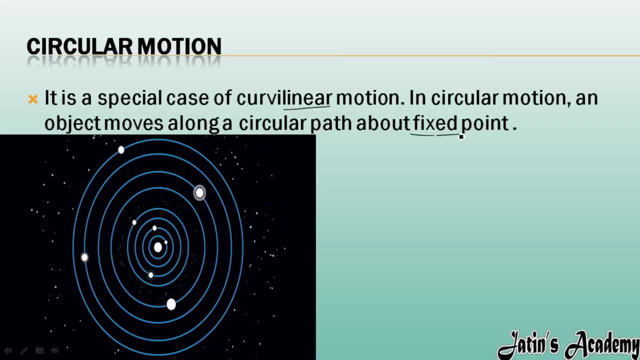 Next we are having circular motion. So what do you mean by circular motion? Circular motion is also a special case of curvilinear motion only, but in a circular motion object moves in a circular path, but about a fixed point of axis. 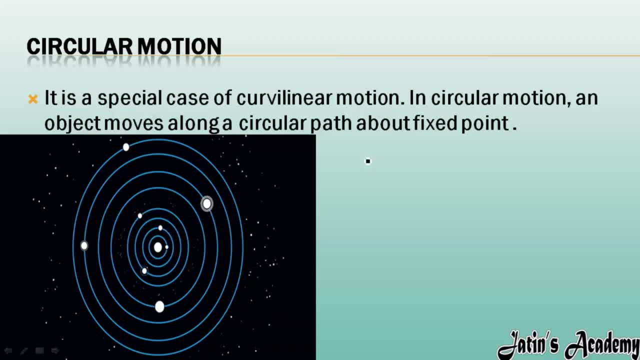 So actually, what is the main difference between circular and curvilinear? Firstly, see what is circular motion. In circular motion, for example, this is a fixed point around this fixed point. This, for example, this boy is running like this around this fixed boy around this fixed point. 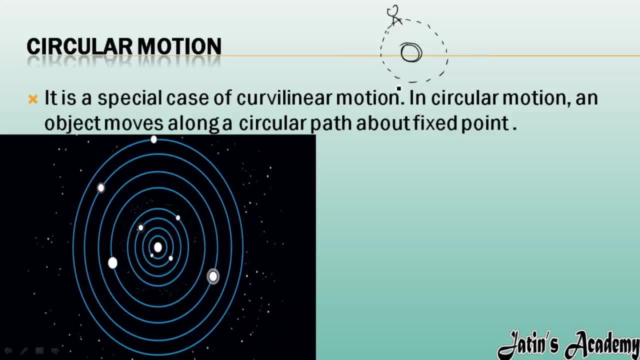 This boy is running like this in a circular motion. So this kind of motion in which object is moving along a circular path, but about a fixed point, about this point only he is moving, He is running in circular path. So this is known as circular motion. 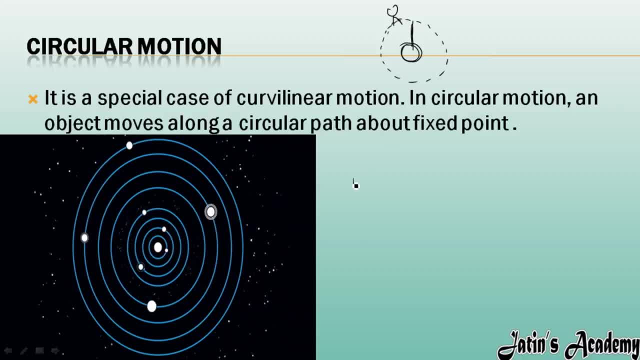 But what do you mean by curvilinear motion? In curvilinear motion, simply object is going in. curve, means in curvilinear motion, No fixed point is there here. in circular motion, One fixed point is there, no. but in curvilinear motion, no fixed point is there. 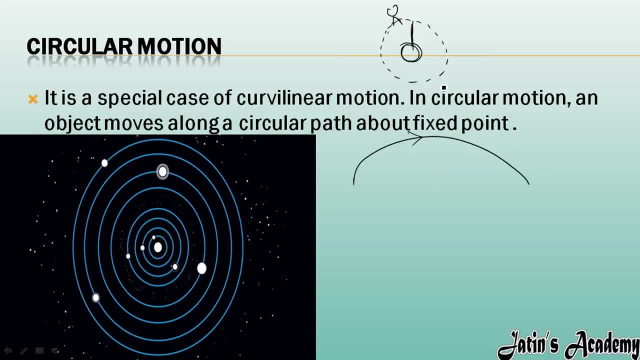 So curvilinear motion. This is the main difference between curvilinear motion and circular motion. Second main difference is this: circular motion repeat itself. It is repetitive in nature. Circular motion is always repetitive in nature. It is also repeating from time to time. 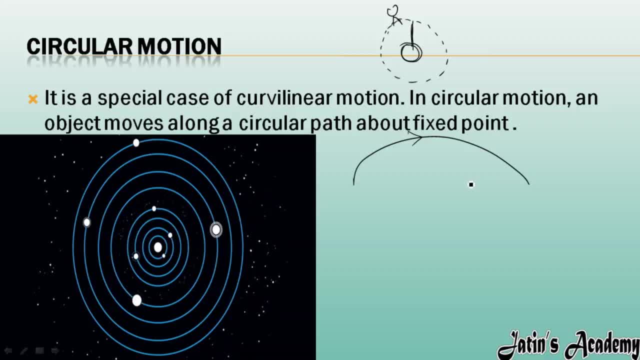 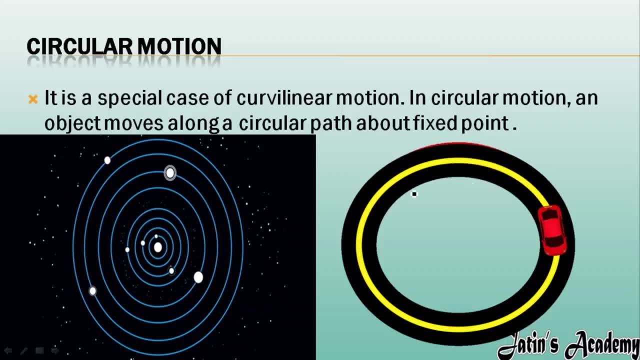 It is repeating like this, but curvilinear is non repetitive in nature. Fine, This is a main difference. So next we are having see, for example, this car is moving along this fixed point. This is a fixed point along which this car is moving. 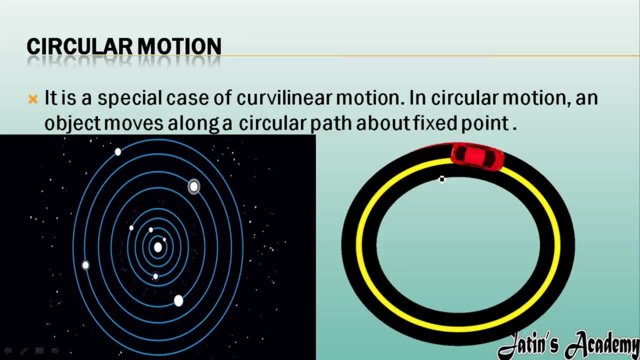 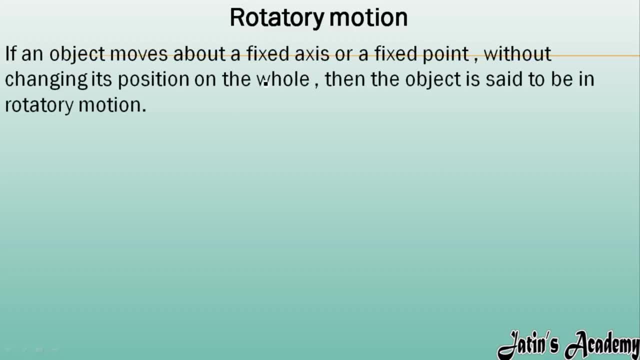 So this car is showing which motion? circular motion. Okay, Next we are having next kind of motion. next kind of motion, that is rotatory motion. So what do you mean by rotatory motion? If an object moves about a fixed axis or a fixed point, but without changing its 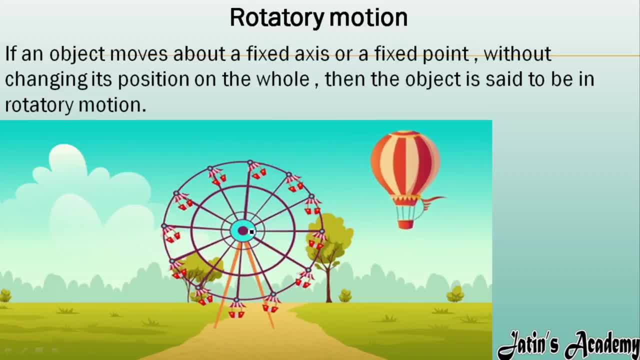 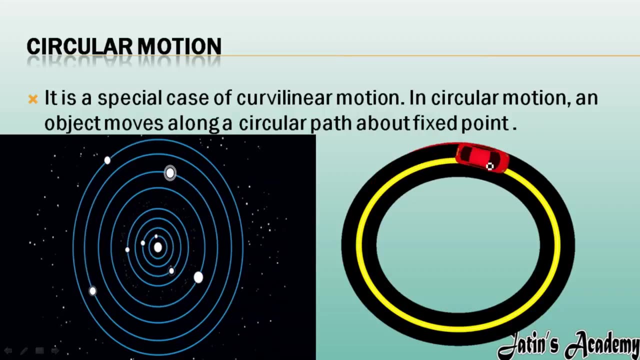 position on a whole. see here, this object is not changing actually its position. This swing is on its like. same position only not like. car is firstly here in circular motion. in circular motion, Firstly car is here, then car full-fledged, changing its position, but here in. 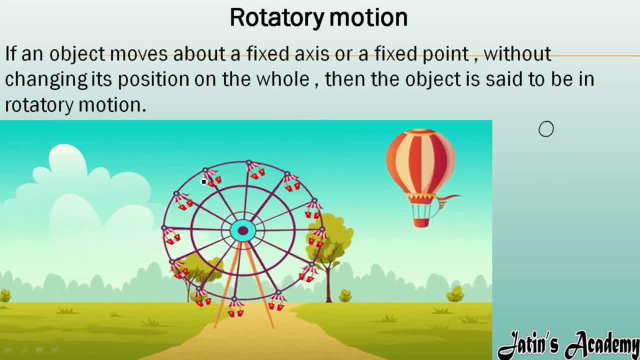 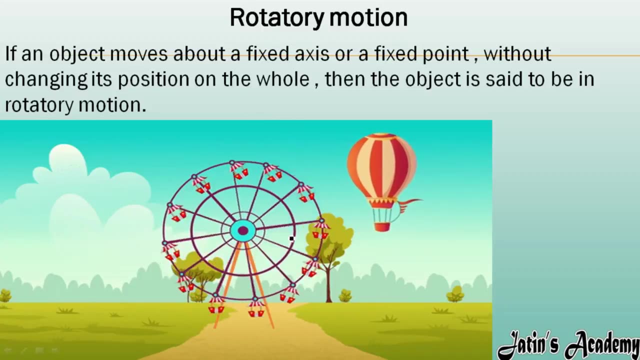 rotatory motion. it is also in only like a circular path only, but here they are not going to change its position. here object is also going to move about a fixed path only, but here object is not changing its position. on a whole object is moving on on a same like path only, same area only, same position only. 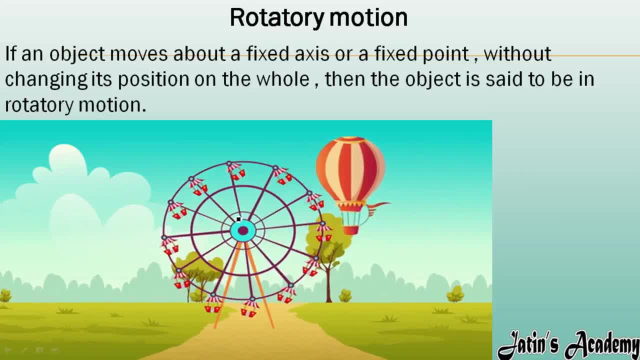 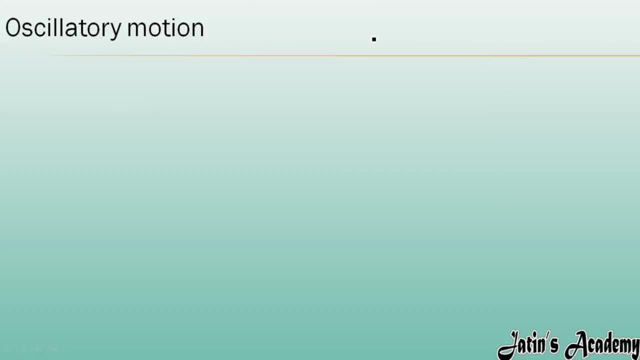 So when object does not changes its position on a whole, but it is moving about a fixed axis or fixed point, that is known as rotatory motion. Next type of motion: We are having oscillatory motion. So what do you mean by oscillatory motion? 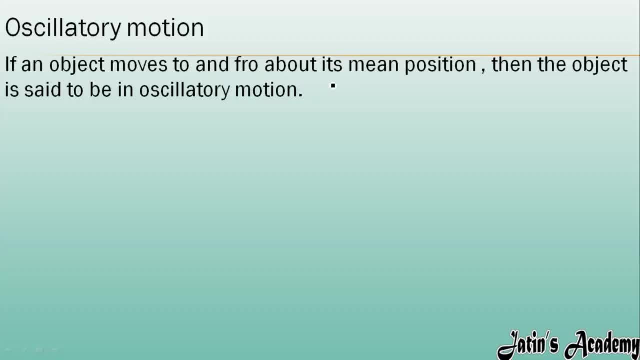 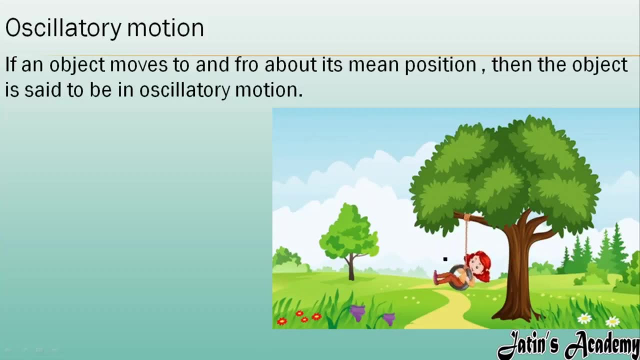 If an object moves to and fro about its mean position, how to and fro see? this girl is moving to and fro like this. to and fro motion is like this: when object is moving like this, like this, or object is moving like this, this motion of an object is known as. 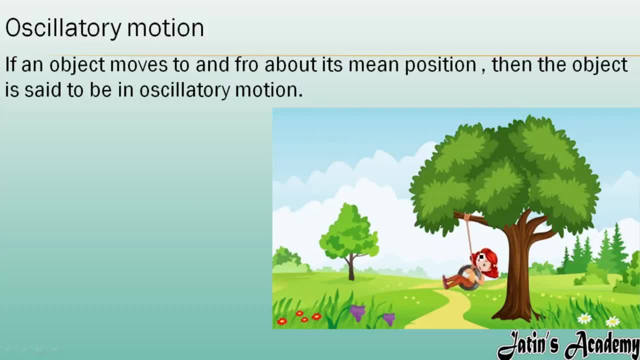 to and fro motion. So this is a oscillatory motion. when object is moving to and fro about its mean position means starting from here till here, So in mean position she is performing, She is moving to and fro, so that motion is known as oscillatory motion. 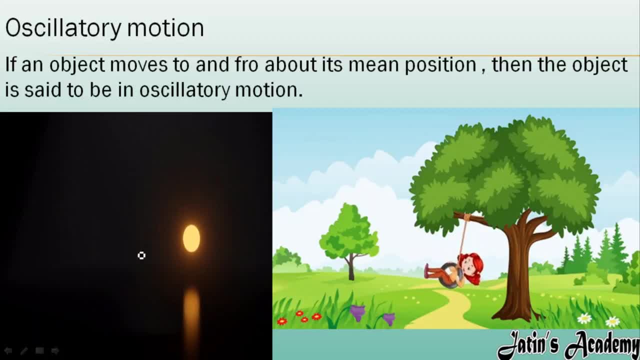 Next example: See this pendulum: when this ball is moving along its mean position, about its mean position, and object is moving to and fro. So what do you mean by Oscillatory motion, when object is moving to and fro about its mean position? 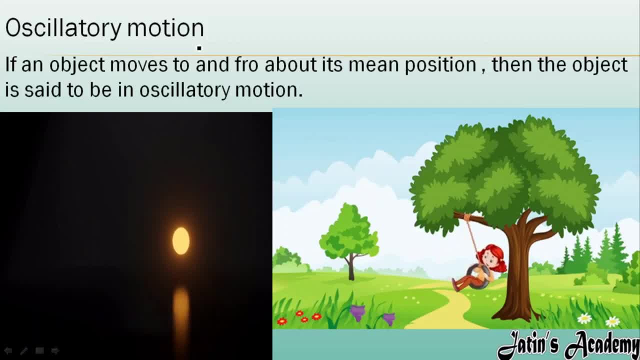 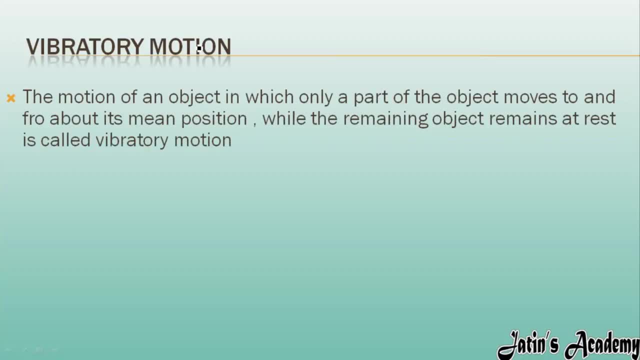 So that object is known as in oscillatory motion. Next we are having vibratory motion. So what do you mean by vibratory motion? The motion of an object in which only a part of the object move to and fro about its mean position, while the remaining object remain at rest. 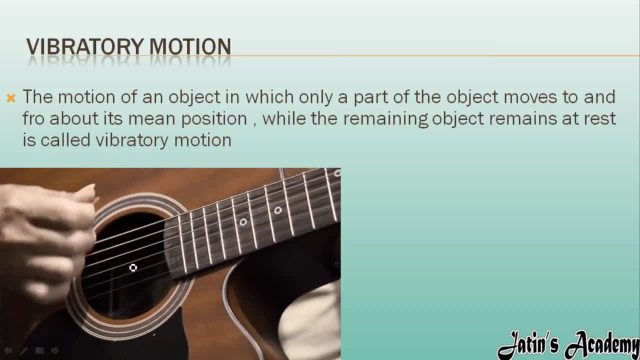 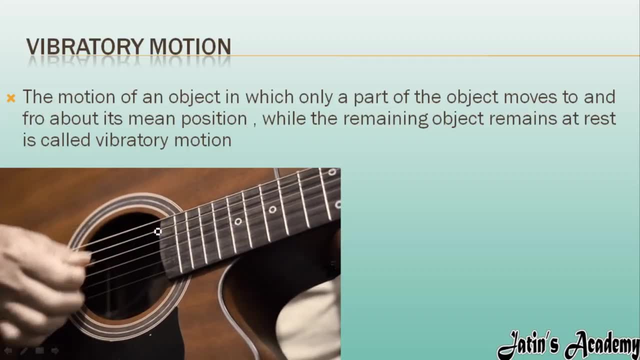 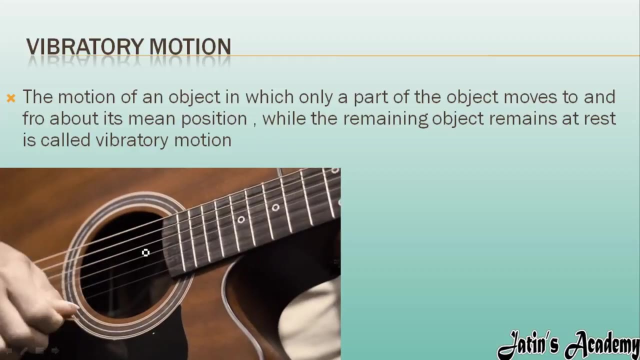 See, for example, here I am having a guitar. in this guitar, When we pluck the strings, this is strings will only move to and fro this, strings are only going to show vibration, but full-fledged guitar is on rest only. so that type of motion in which, like few, part of the object is in vibratory motion or few. 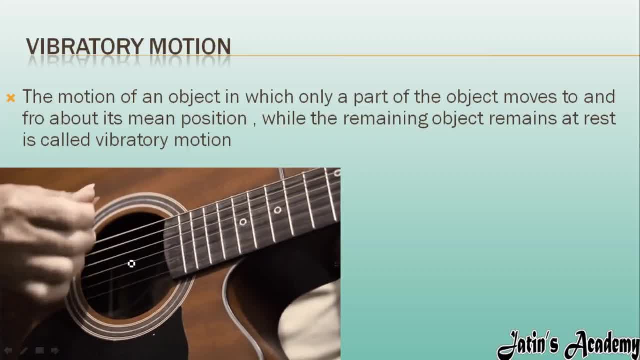 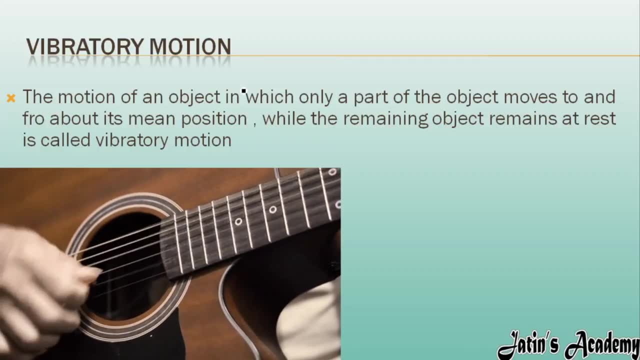 part of the object is showing to and fro motion about its mean position, while the remaining object is in the rest. so that type of motion is known as vibratory motion. For example, beating of this membrane of drum. when you will beat the membrane of drum membrane. 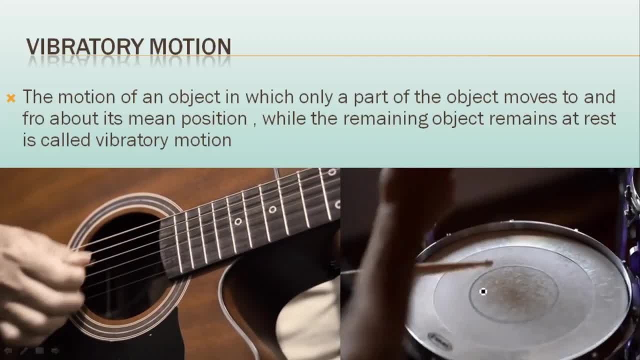 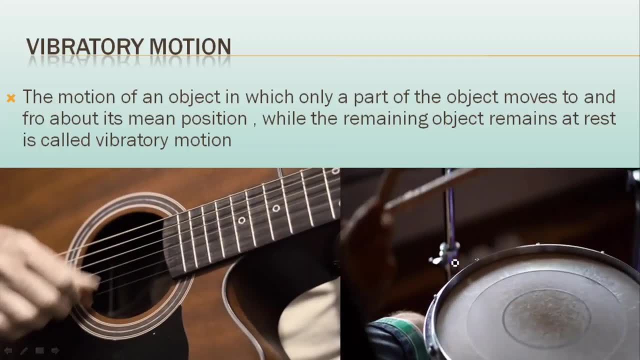 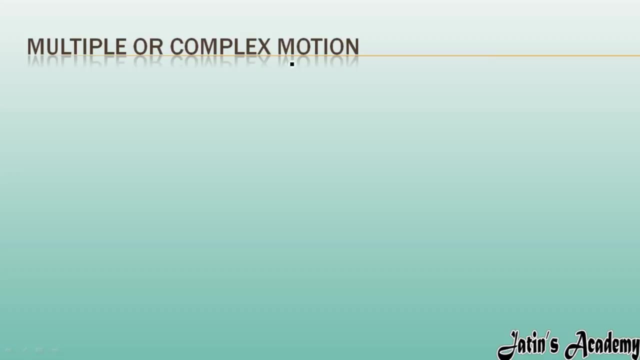 means this white portion. So when you will beat the membrane of drum, only the membrane of drum will show to and fro motion, but rest of the drum is in, rest only. So this kind of motion is known as vibratory motion. Next we are having multiple or complex motion. 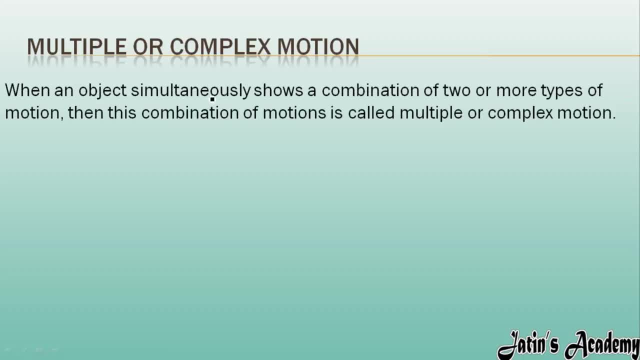 So what do you mean by multiple or complex motion? when an object Simultaneously show a combination of two or more type of motion means when one object is showing two or more types of motion. For example, this biker is moving in a straight line due to the movement in straight line. 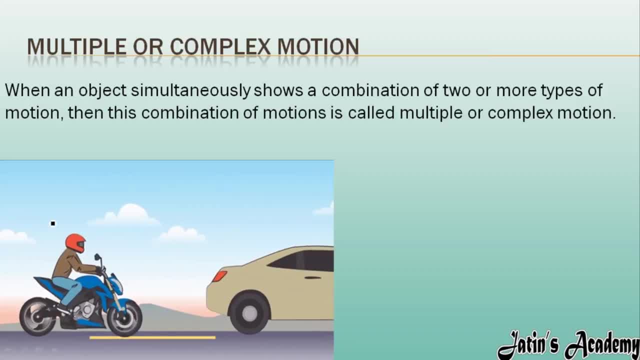 which motion is there? Yes, it is rectilinear motion. So when biker is moving in a straight line, their rectilinear motion is there. plus these wheels of the car, wheels of sorry wheels of this bicep wheel of this motorcycle, They are also rotating about the fixed position. 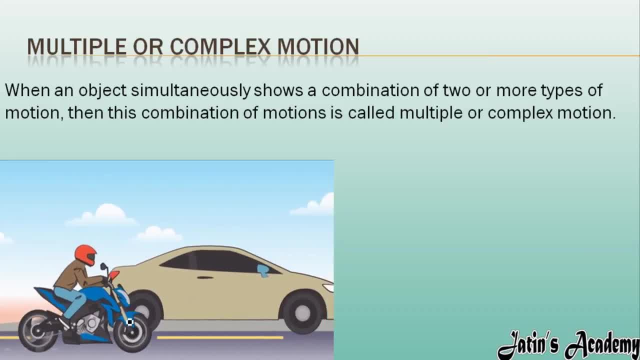 So that is known as rotatory motion. So this biker is showing two or more kinds of motion, that is, it is showing rectilinear motion also, rotatory motion also. So when one object is showing the combination of two or more type of motion, then this combination 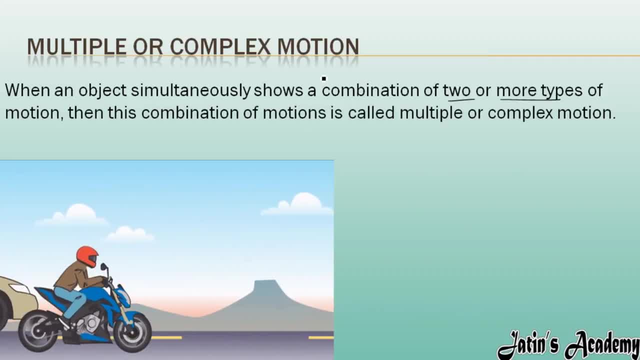 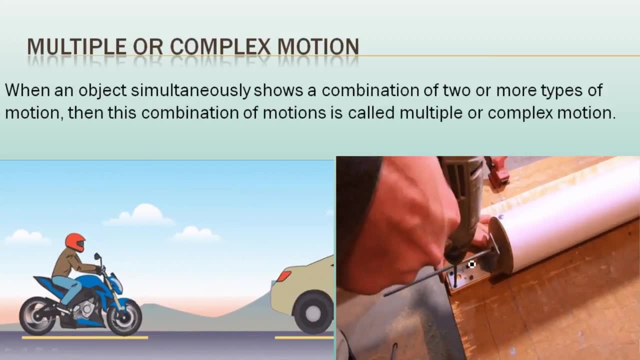 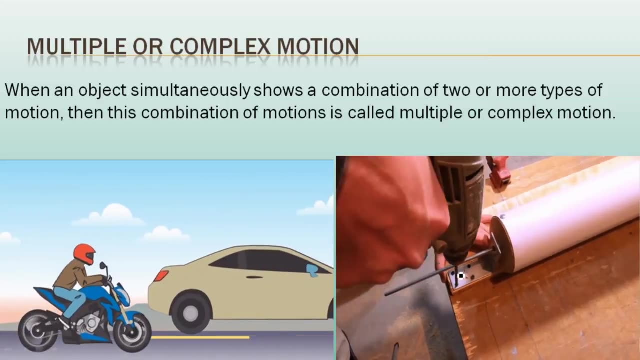 of motion is known as multiple or complex motion. Any other example you can see, for example this drilling machine. this drilling machine is showing downside also means rectilinear motion, plus it is rotating also. this machine is rotating also, so that machine is in the rotatory motion also. 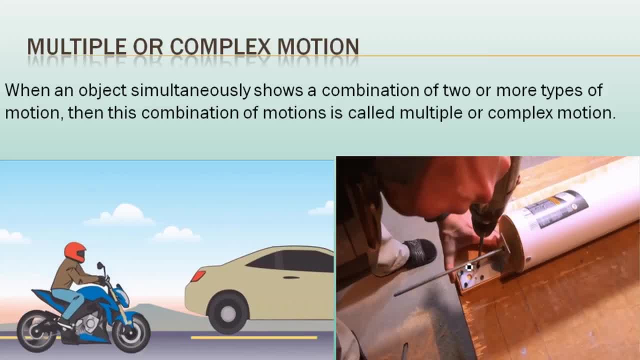 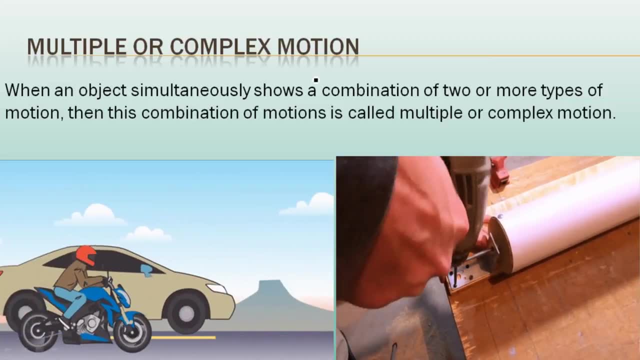 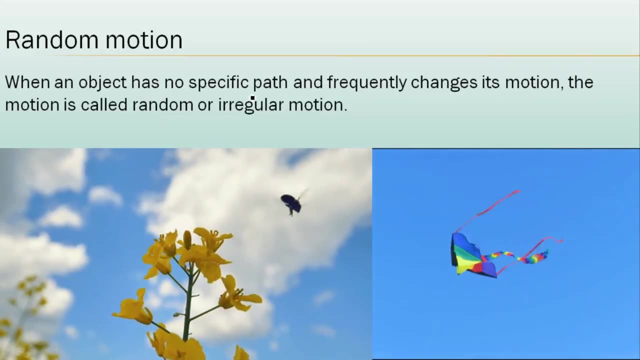 So when one object, one, this drill machine, is showing two kinds of motion at the same time, that combination of motions is known as multiple or complex motion. Next, we are having random motion, as a name suggests, random. random means when an object is not having its specific or particular path. specific means particular path: when an object is not having 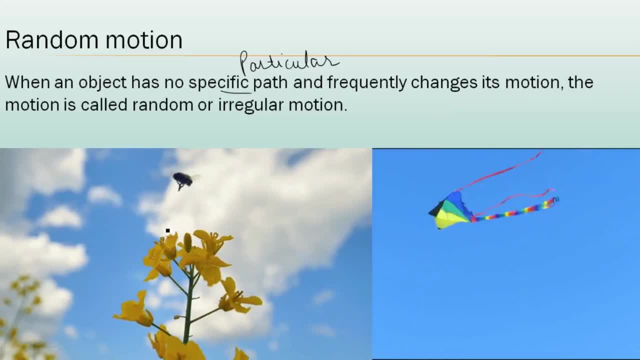 its particular path and frequently changes its motion, like this B See this insect is randomly moving here and there means this insect is not showing a single type of motion. firstly is she is coming here, then going back, So when object is not having a specific path and frequently changes its motion, like this kite. 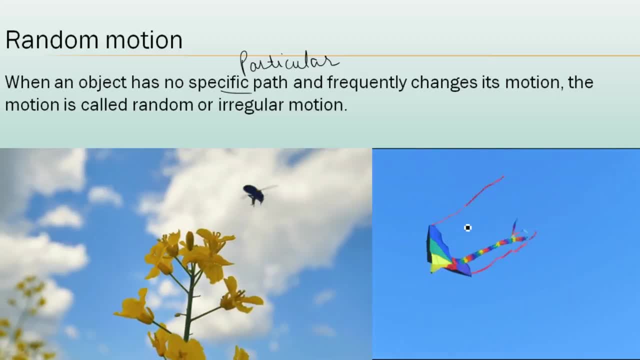 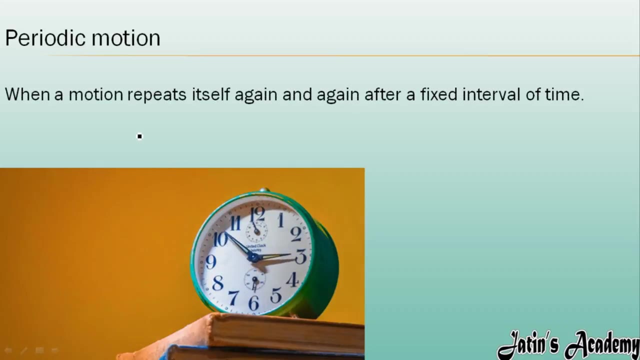 kite. So kite is also not Having its particular path, so it is also changing its motion. So that kind of motion is known as random or irregular motion. fine, Next we are having periodic motion. What do you mean by periodic motion? when a motion repeats itself again and again after a fixed interval. 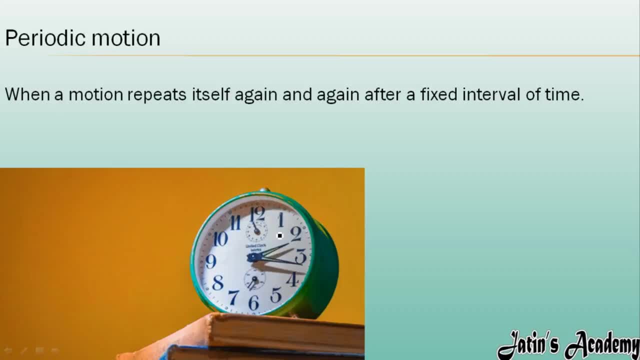 of time when a motion is repeating itself means, for example, these hands of the clock, these hands of the clocks are changing or repeating It's motion again and again after fixed interval of time, like firstly 3 o'clock, then afterwards also after 12 hours, then again 3 o'clock, then again 3 o'clock. hands of the clock is also means repeating itself. 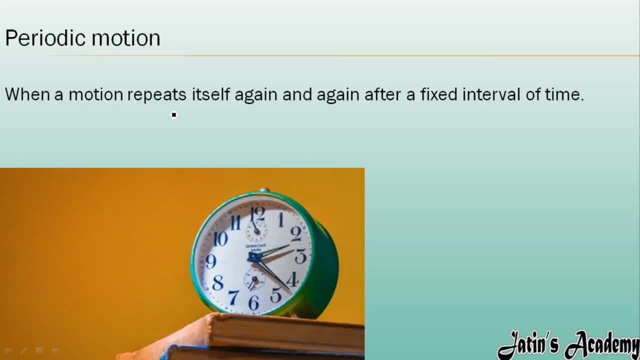 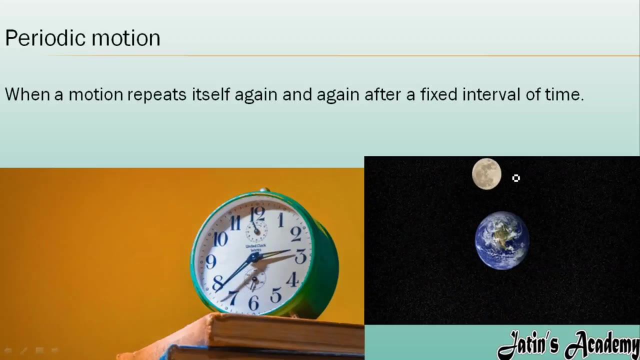 again and again, So that motion in which object or in which object is showing motion which is repeating again and again after a fixed interval of time. that motion is known as periodic motion. For example, rotation of the moon around the sun, so rotation of moon around for the earth, rotation of moon around the 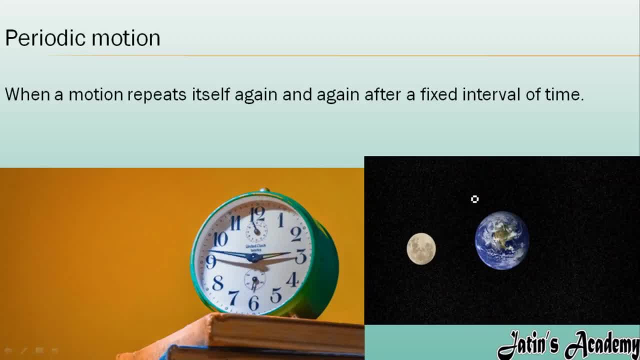 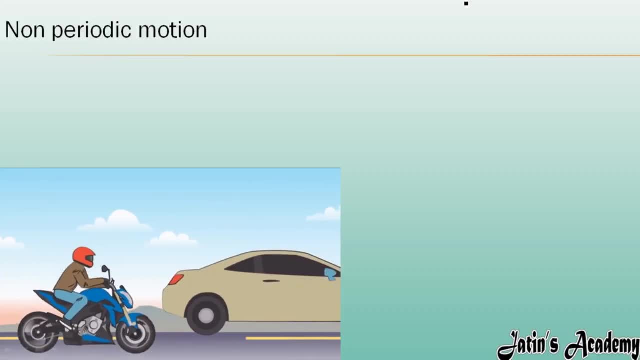 earth is also a periodic motion which is repeating itself after a regular intervals of time. fine, Next we are having non-periodic motion. So what do you mean by non-periodic motion, when a motion does not repeat itself after a regular intervals of time? for example, this biker is here on this road. 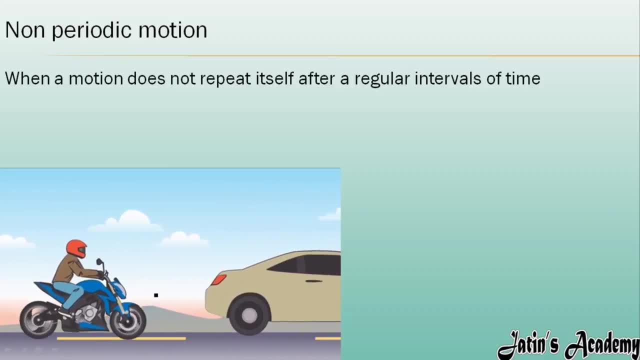 But after 1 hour, after 2 hour again, he will come here. only know so when a motion does not repeat itself again and again after fixed intervals of time, so that motion is non-periodic motion, like in a case of hands of clock, it is obvious. 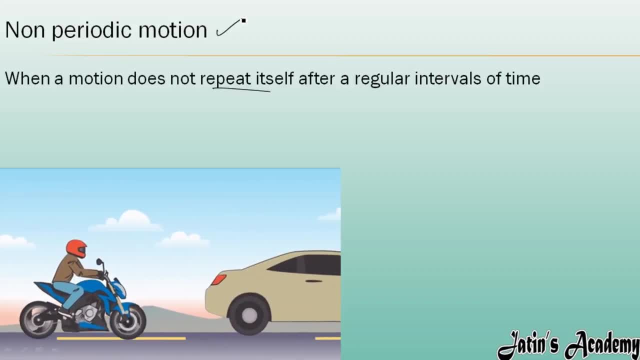 It is sure that hands of clock will again come to their position after fixed intervals of time. that is why it is a periodic motion. but here, in non-periodic motion, object does not repeat its motion after fixed regular intervals of time, So that motion is known as non-periodic motion. 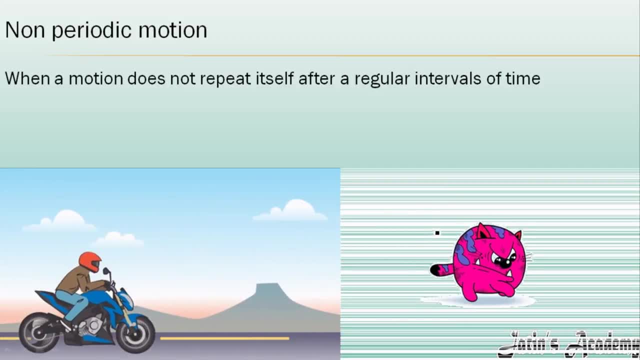 Say this movement of cat. firstly, cat is there in your house. Okay, today she came, but tomorrow it is sure she will come again, or day after tomorrow sure it will come again. No, So when object does not repeat itself after regular intervals of time, that motion is a non-periodic motion. 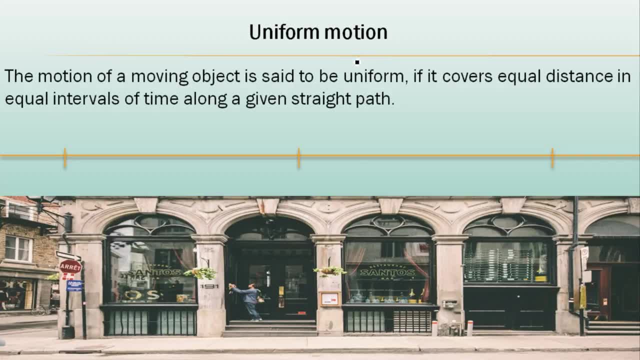 Next, we are having uniform motion. So what do you mean by uniform motion? a motion of an moving object. Object is said to be uniform If it covers equal distance in equal intervals of time. how, for example? see this example. first, This car is moving. 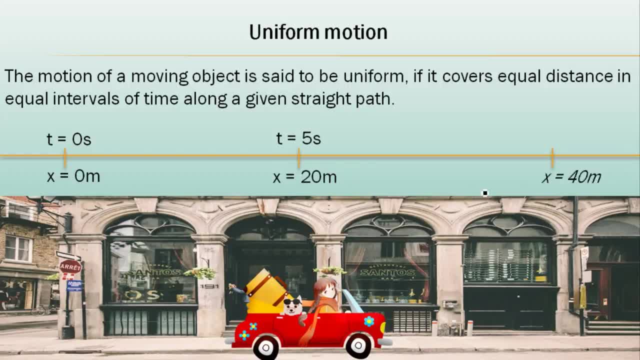 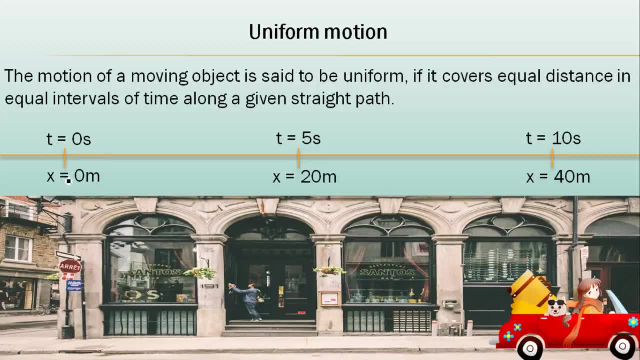 Then again it come to this point Afterward. this come to the last point here. fine, So what is happening here? firstly, car is there on this point where distance is 0, time is 0 means car has to start. at this point where distance is 0, time is 0.. 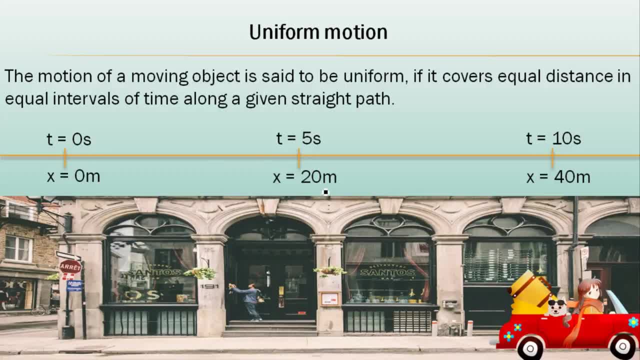 So after 5 second car covers 20 meter. after 5 seconds this car covers 20 meter again after 5 minutes. See here: 5 second is there, then 10 second is there. What is the gap between these two times? gap is 10 second minus 5 second, that is, gap is of 5 second. 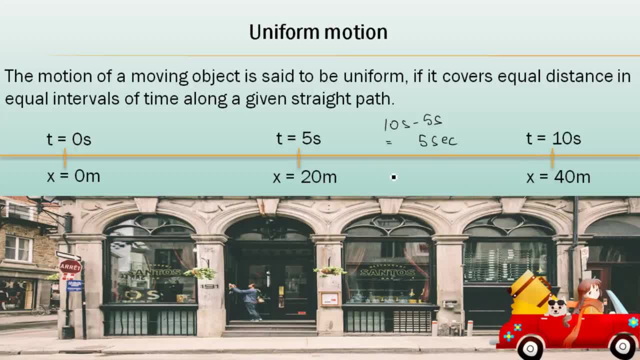 So after again 5 second it covers how much distance. again you can see distance. here is 40 meter. here distances 20 meter. So it covers How much distance: 20 meter again. So when object is moving same distance in equal intervals of time here. here also you can see when car. 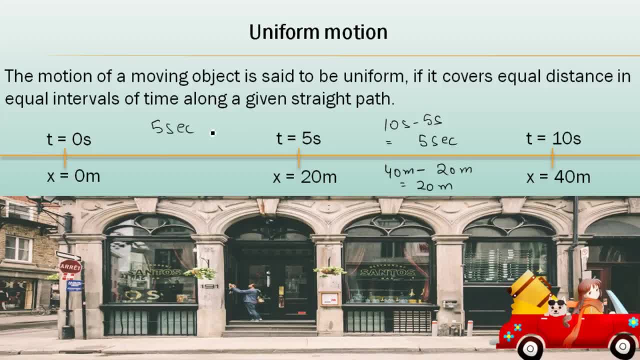 is at 0 second. in 5 second it reaches at point B. This is point A. This is point B. This is point C. in 5 second It's reached at point B. and how much it covered. it covered 20 meter. 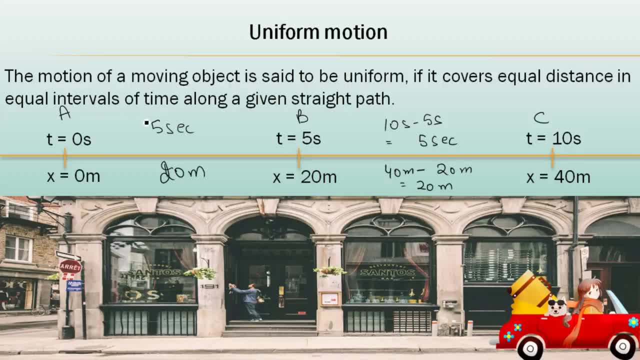 Fine. So here in 5 second from A to B. in 5 second Car covered 20 meter. again from B to C. It takes 5 second only to cover 20 meter. So when object is moving and object is cover equal distance in equal intervals of time, that motion is known. 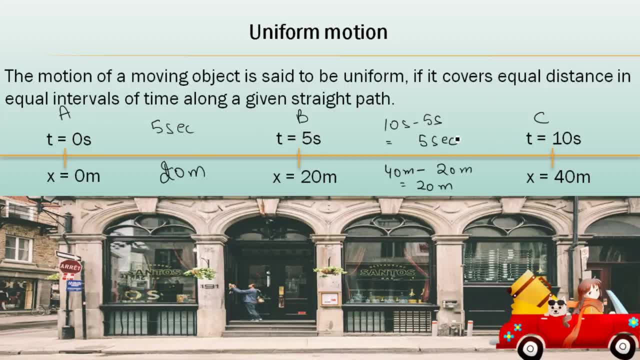 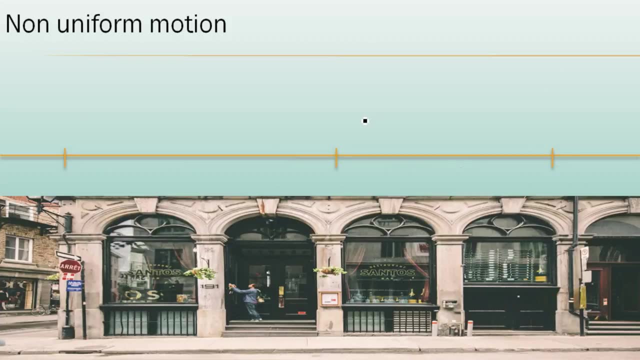 as uniform motion clear might be. this is clear to you. when object is moving, when object is covering equal distance in equal intervals of time, that is known as uniform motion. but uniform motion always takes place along a straight path. Fine. Next we are having non-uniform motion. 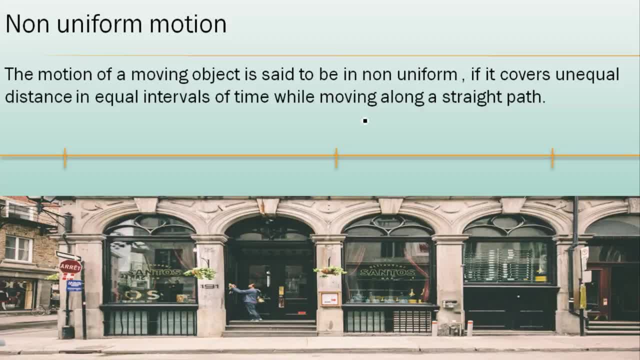 So what do you mean by non-uniform motion? The motion of an object is said to be non-uniform if it covers unequal distance in equal intervals of time. unequal distance. See, for example, this car is firstly here, then it comes toward point B. 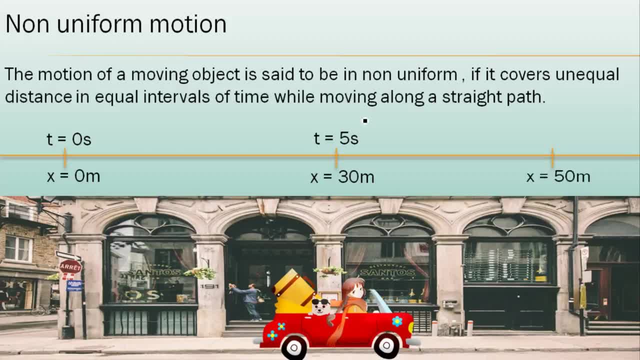 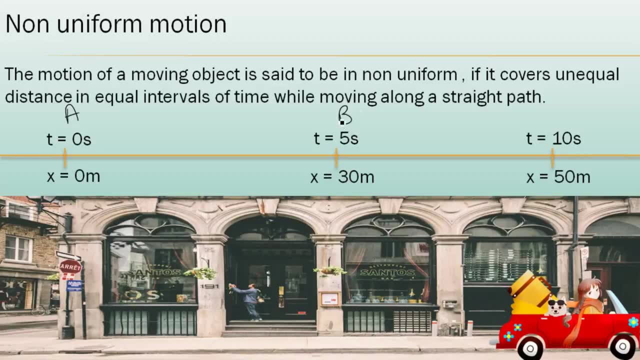 Finally, it comes toward point C. It is coming toward point C Now, Yes. So now let us see here, from point A, B, then point C, from point A to point B, How much time it covers here It is 0 second here. 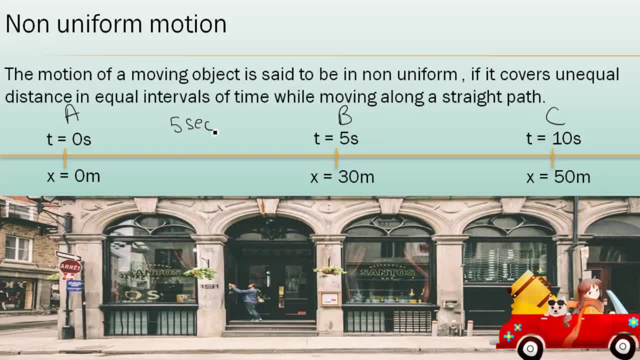 It is 5 second. So what is the time covered here? 5 second. here it is 0 meter, here 30 meter. So here it covered 30 meter. So this car covers 30 meter in 5 second. now see from point B to point C, from point B to point C, how much. 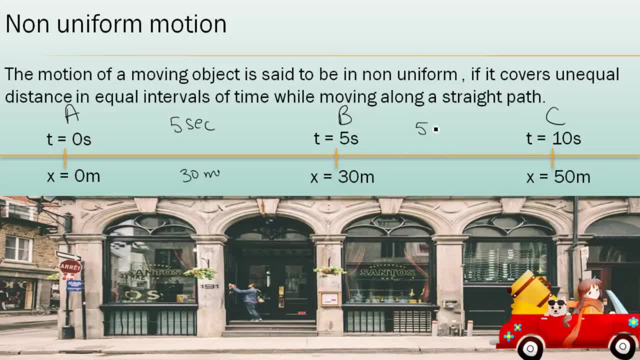 time it took 5 second to 10. second means how much gap, 5 second gap, Then it covers 30 meter to 50 meter. How much distance it covered, that is 20 meter. Now you can see in 5 second. firstly car is covering 30 meter, then again in 5 second. 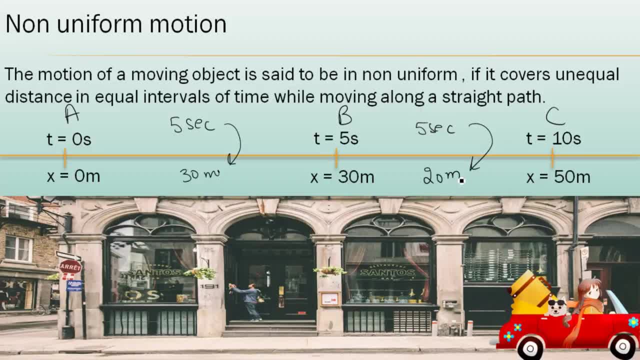 But now it is covering 20 meter might be in between traffic is there. That is why distance covered is less so. non-uniform motion means when object covers unequal distance in equal intervals of time. Actually, time is equal only, but here distance is unequal. 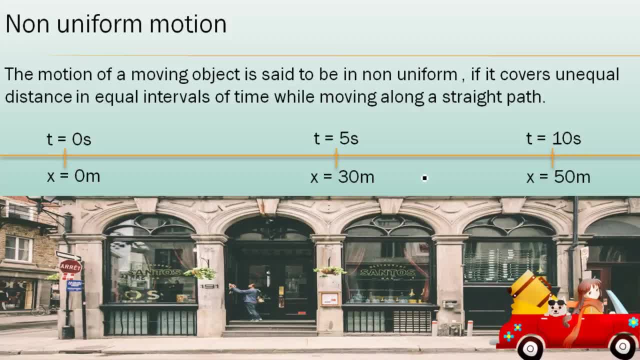 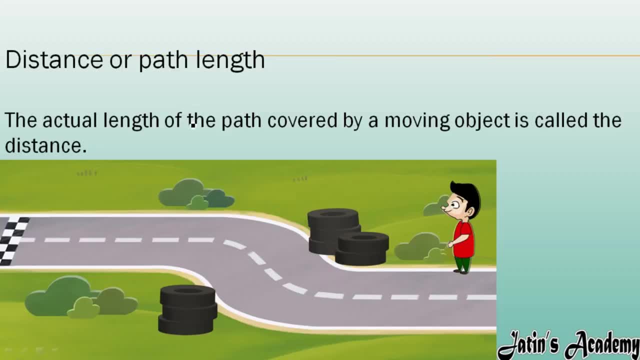 So it is known as non-uniform motion. Next, we are having distance or path length. So what do you mean by distance? the actual length or the path covered by a moving object is known as distance. whatsoever is a actual path. Now this boy wants to go from this point, from this point. 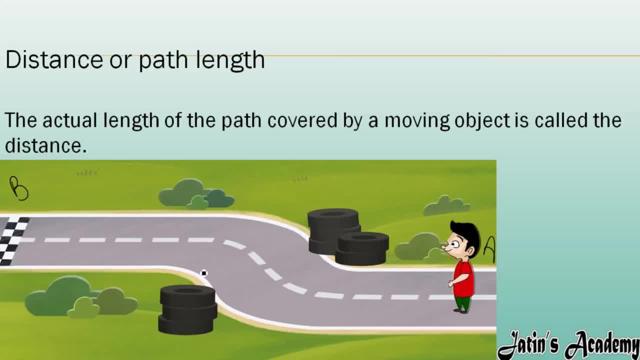 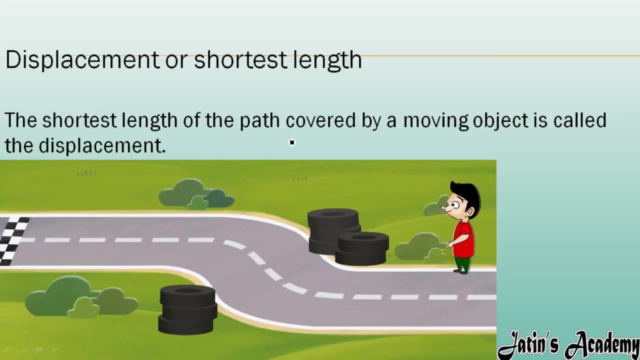 A to, at last, point B. So whatsoever distance this boy is going to cover, that distance is known as Path length or distance. this actual length, whatsoever, This actual length is covered by a by this boy. that is known as its distance. fine, Next we are having displacement. 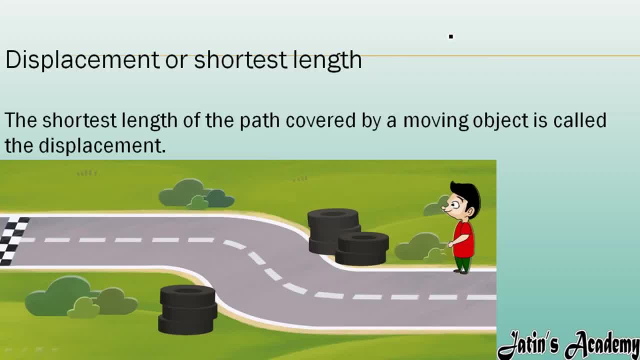 What do you mean by displacement? I will give you one simple example, For example. this is a path. This path is having point A, B, C, D. fine, Here one boy is standing. boy wants to go from point A towards point D. So how he can move from point A to point D, two methods are there. 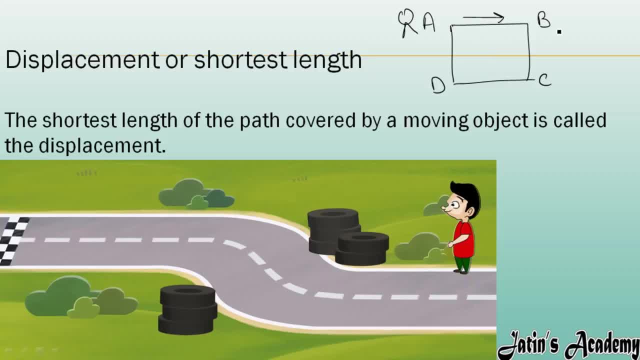 Firstly he can go from point A to point B, Then he can move from point B to point C, afterwards from point C, Then finally at point D. This is the first method. So in this first method actually he has covered actual path, full distance. 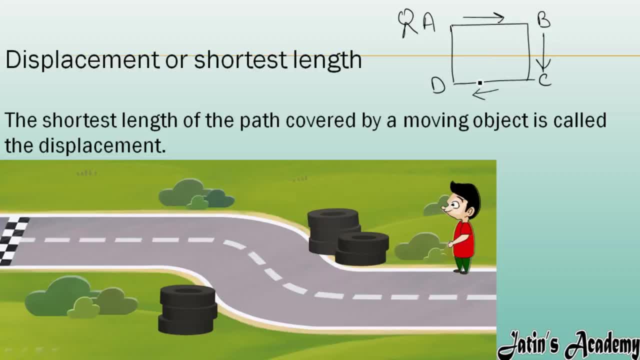 He has covered actual path He has covered, so that is known as distance traveled by him. This boy, in this case, has covered distance. But second method is also there in order to reach from point A to point D directly. He can come from point A to point D like this shortcut: 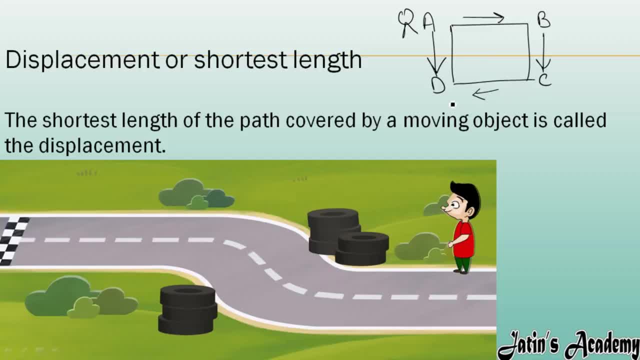 He can take or no. So this total length covered by a body is a distance, And the shortest length covered by a moving object is known as displacement. This is the main difference between distance and displacement. Now see how this boy will move from here. 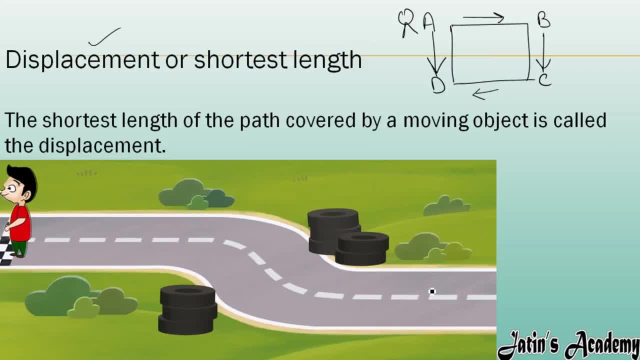 So without going here, So without going to this way, he is directly going in a straight way, So he is covering the shortest length. So it is the actual main difference between the distance and displacement. So next we are having one numerical related 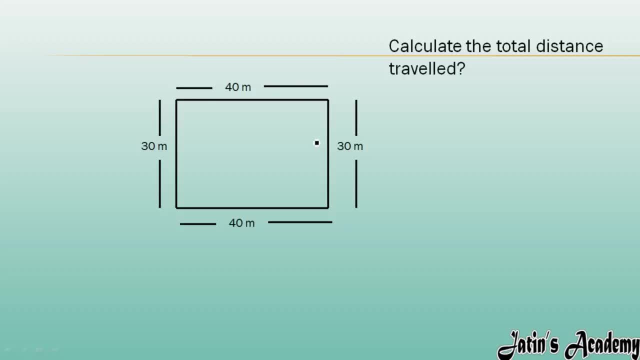 To the distance. calculate the total distance of this path. For example, this boy is standing here at point A, He wants to go till point A again. Firstly, standing at point A, He wants to go again at point A. So how he will move, firstly, 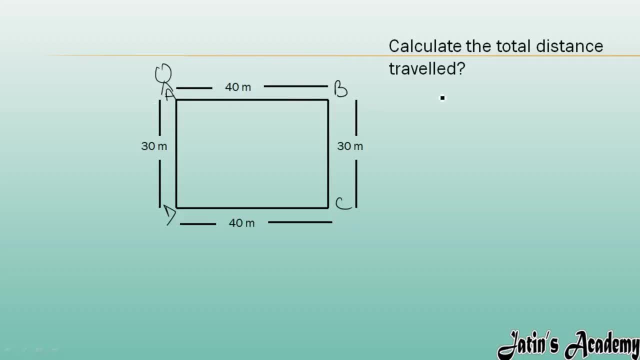 He will go from point A to point B. from point A to point B, How much distance? 40 meter plus. then from point B to point C: 30 meter. Then from C to D: 40 meter, then again from D to A, that is 30 meter. 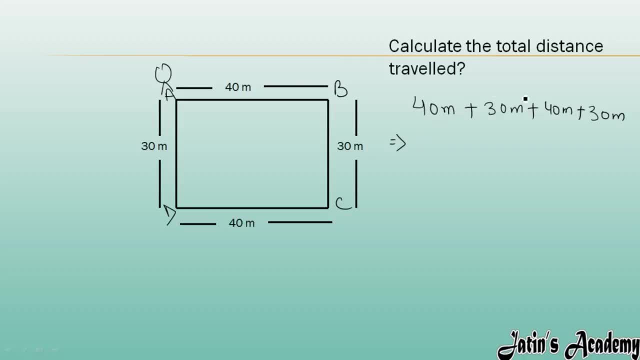 So how much distance he has covered: 4 plus 4, 8, that is 80 meter. plus 3 plus 3, that is 60. 30 plus 30, that is 60.. So how much distance he has covered: 140 meter. 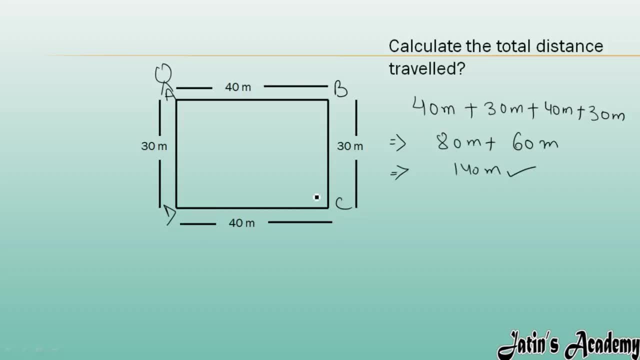 So this is a total distance traveled by a object. Okay, So next we are having: Distance is a scalar quantity. Now we will see that. what is the difference between scalar and vector quantity? Firstly, I want to tell you what is the difference between scalar. 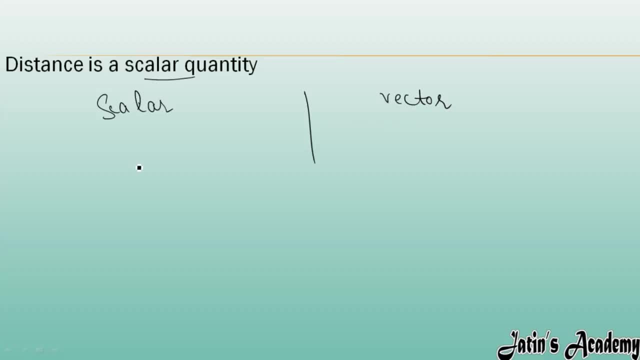 And vector quantity. So what is scalar quantity? scalar quantity is that quantity which is having only magnitude. Scalar quantity is a quantity that is having magnitude But no direction. here in scalar quantity We will not bother about direction, We will only see the magnitude. magnitude means for example, like a boy covers 40 meter. 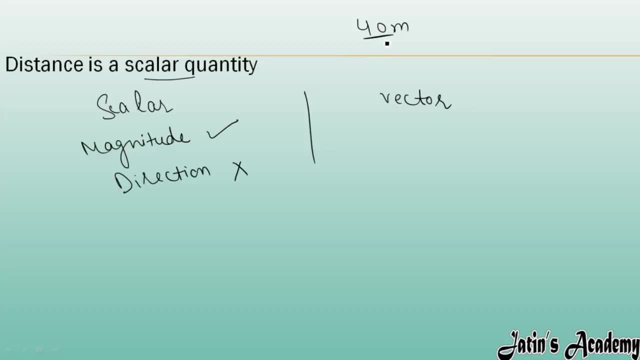 A boy covers 40 meter. here magnitude is 40. how much distance he has covered 40 meter? So magnitude we are watching, but in which direction he has moved, that is not our tension. Okay, So in scalar quantity we are only checking magnitude, but no direction. 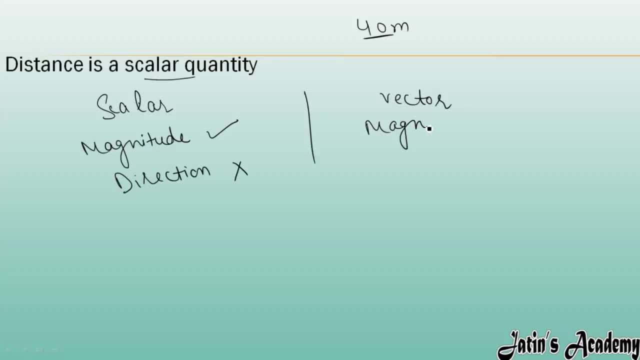 But In the vector quantity we are checking both. We are taking care of both things, about magnitude as well as direction. So what do you mean by scalar quantity? scalar quantities are the quantities in which magnitude we are watching, in which there is a magnitude but no direction. 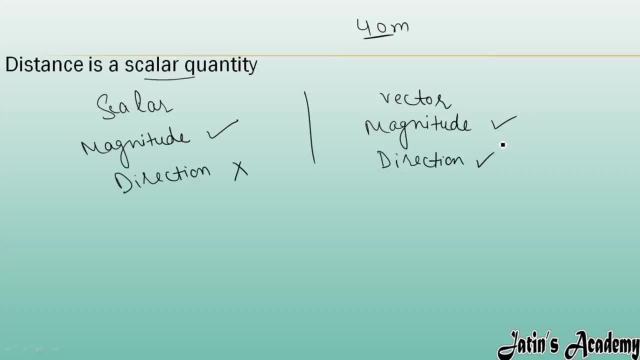 But in a vector quantity there is magnitude as well as direction. So now we will do: distance is a scalar quantity. distance is a scalar quantity means in distance We will only take tension of magnitude. We will not see the direction, that in which direction that boy moved, that is not our problem. 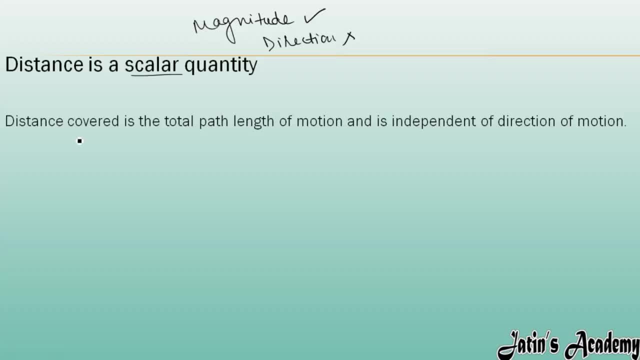 So we will see only magnitude. distance covered is a total path. length of motion is independent of direction of motion. So distance will not dependent upon motion. this distance will not take care of the direction. distance will only take care of the magnitude. So here we are having pictorial representation. 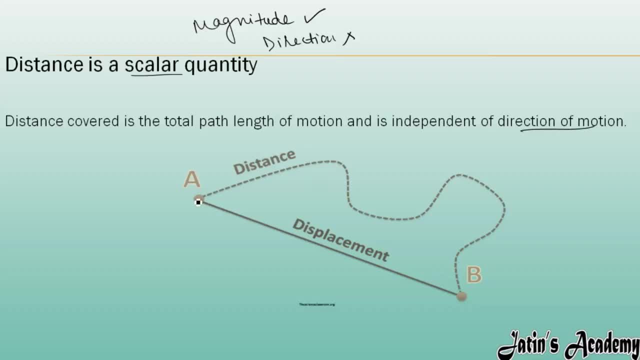 If body wants to move from point A to point B, So this is the actual path. Firstly he will go here, then here at last, point B. So this is the actual path covered by a body and this is the shortest part, that is a displacement covered by a body here. 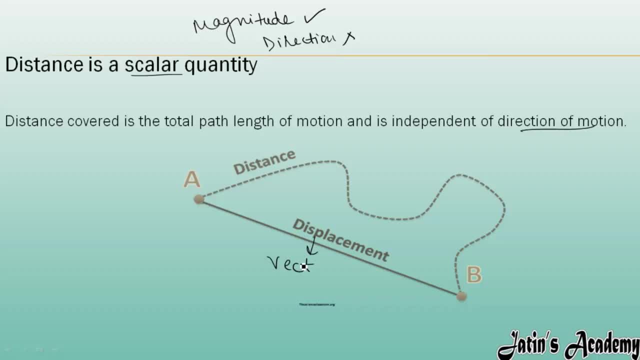 Distance is a scalar quantity, but displacement is a vector quantity. vector quantity means in which we are watching both magnitude, in which we are bothering about Both magnitude also, plus direction also. Okay, at which direction he is going? in which direction? from point A to point B. 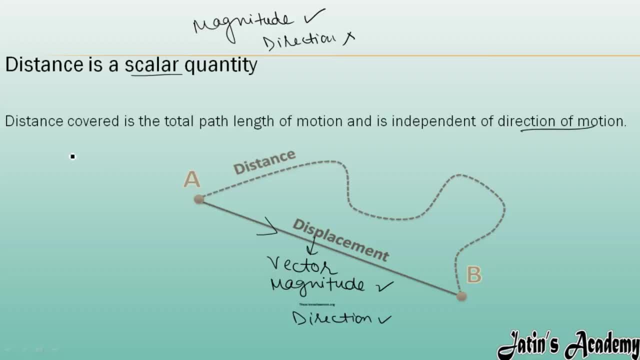 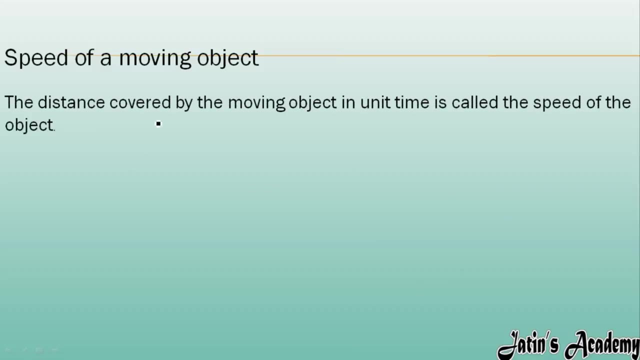 Obviously has to go this direction. only if he will go to backside how he will reach to point B. fine, So displacement is a vector quantity and distance is a scalar quantity. So next we are having speed of a moving object. So what do you mean by speed of a moving object? distance covered by a moving. 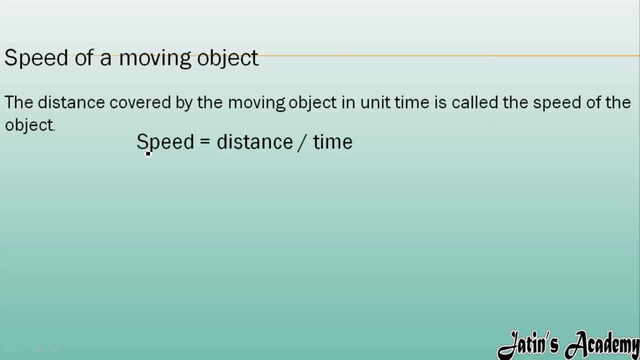 Object in unit time, how much distance object has covered in how much time. for example, this is a object, So this much distance that object has to cover in a time in particular, time, So that distance over time will give you speed. So distance covered by a moving object per unit time is known as its speed. speed is equals to distance over time. 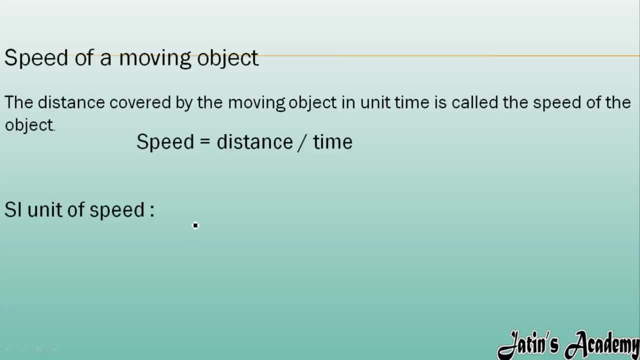 Now we are having SI unit of speed. We are going to calculate the SI unit of speed. So we know here: SI unit of distance. Firstly we will see the SI unit of distance. So SI unit distance is what meter? and SI unit of time is second. 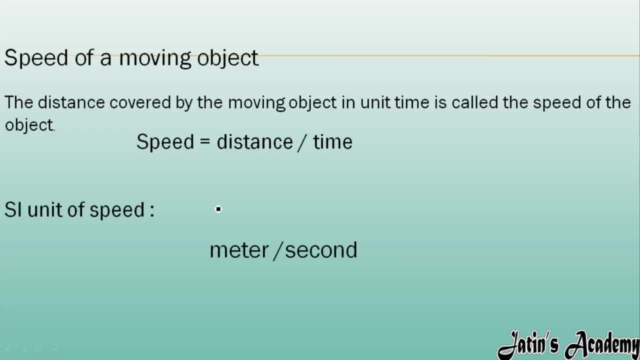 Okay, so we will see firstly SI unit of distance, then we will see SI unit of time. So now the SI unit of speed is meter per second. You can write like this also. You can write like this also: SI unit of speed is: 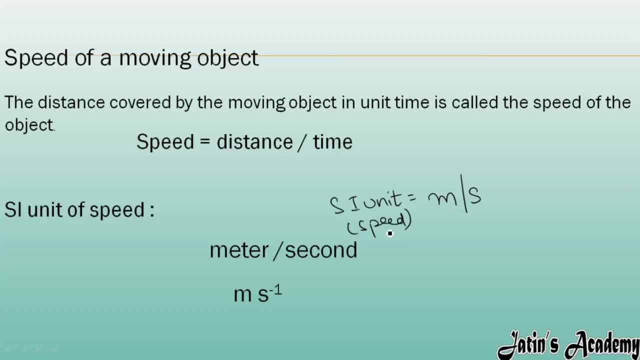 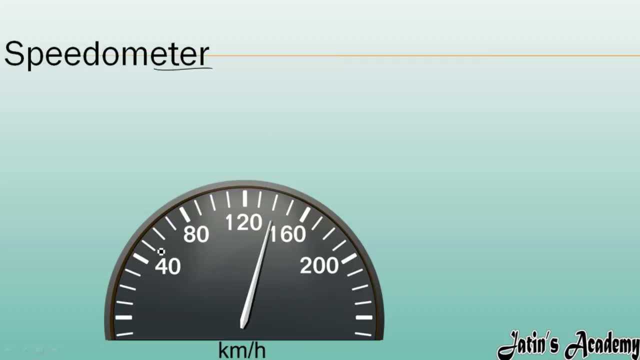 SI unit of speed is meter per second, fine. Next we are having speedometer. might be you have seen this kind of instrument installed in our like activas or installed in our car. So what do you do? What do you mean by the speedometer? speedometer is a fitted in car as well as in motorbikes. 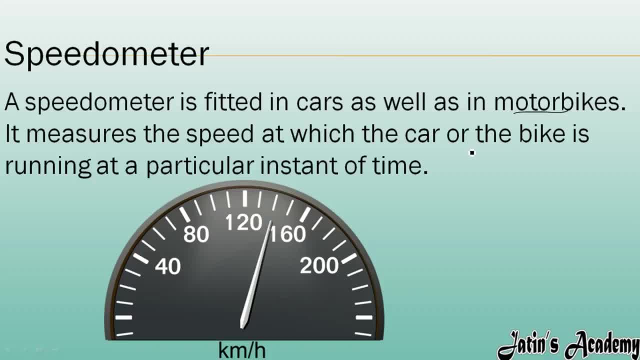 Actually, speedometer is a device that is used in a car or bike to check the speed of a car, Speed of the running car at a particular instant of time. So speedometer is fit in the car as well as motorbike and it measures the speed of car or bike at particular instant of time. 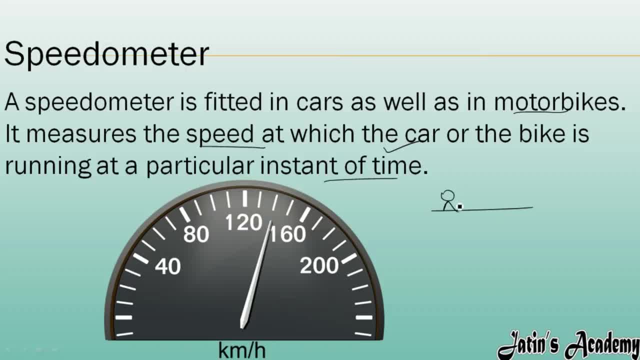 Like, for example, I am riding my activa and I want to see what, at what speed, I am going. So to check, in order to check at what speed I am going, I will see the speedometer. So speedometer will give me the reading. 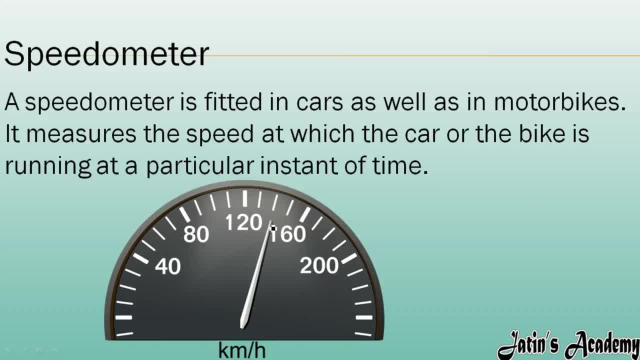 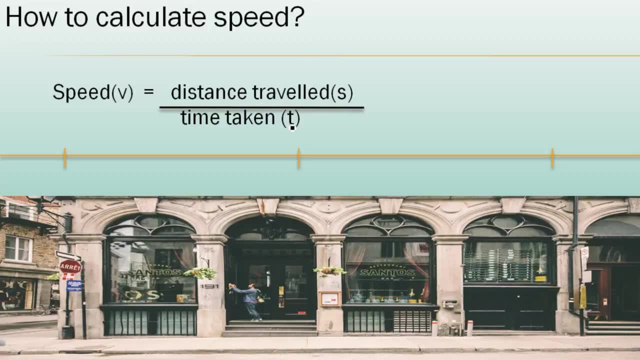 That at what speed my activa is going? fine, How to calculate speed. So we have already discussed the formula of speed, that is, speed is equals to distance upon time. So by this formula we can easily calculate the speed. for example, This car is firstly on point a afterwards. 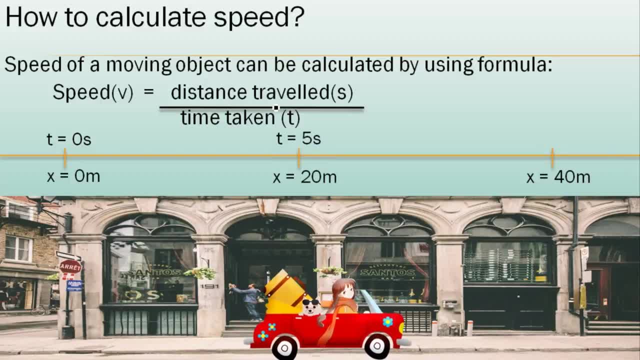 It moves toward point B, then again it moves toward point C. So at this point C, I want to check that. what is the speed of this car? fine, So what is the speed? actually, speed is distance over time, How much distance this car has covered. 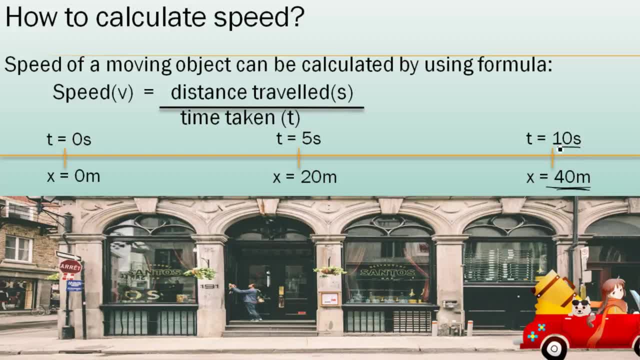 So this car has covered 40 meter. in how much time? in 10 second It has covered 40 meter. So what do you mean by speed? speed equals to distance. distance, that is 40 upon time. time is 10.. So speed of this car is 4 meter. 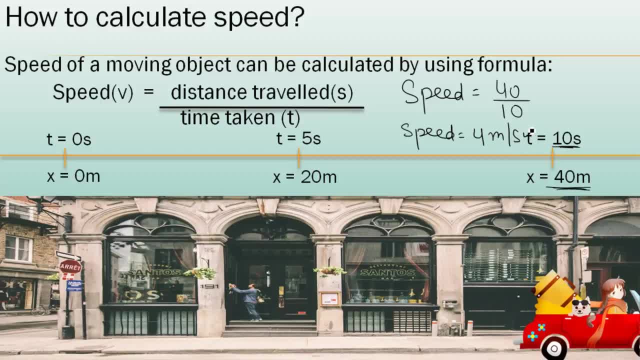 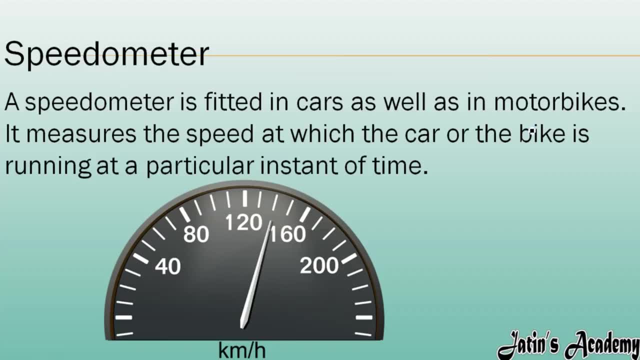 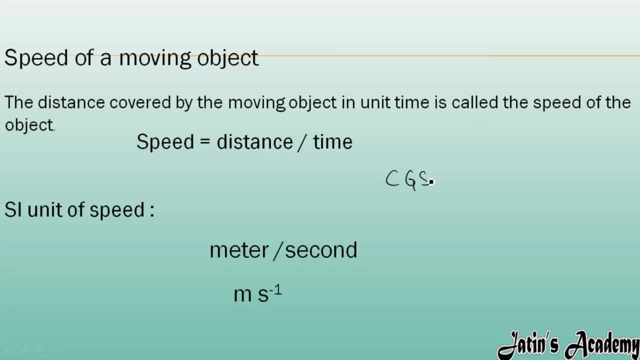 Second, clear speed of this car is 4 meter per second. One thing more in the speed topic: here We have discussed about the SI unit of speed. here I want to tell you about the CGS unit of speed, also CGS unit of speed. 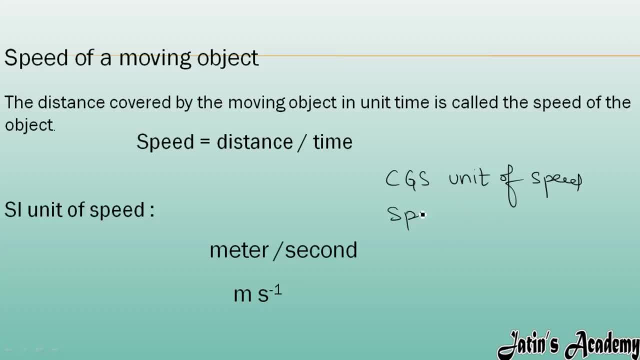 So see how to calculate CGS unit of speed. We know speed equals to distance upon time. Fine, So here distance is what in CGS actually we are having. C means centimeter, G means gram and S means second. S means second. Okay. 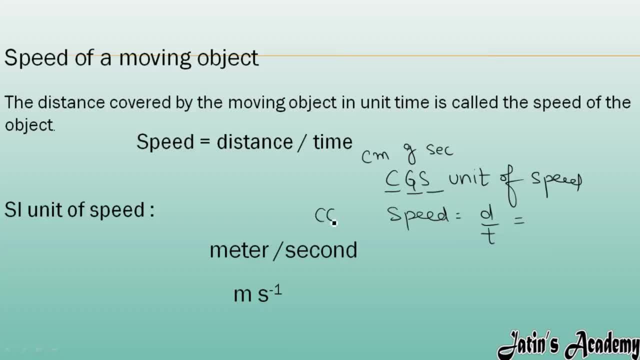 So here we want to check the CGS unit of speed, CGS unit of speed. So tell me what is the CGS unit of distance? CGS unit of distance is centimeter and CGS unit of time is second. So CGS Unit of speed is centimeter per second. 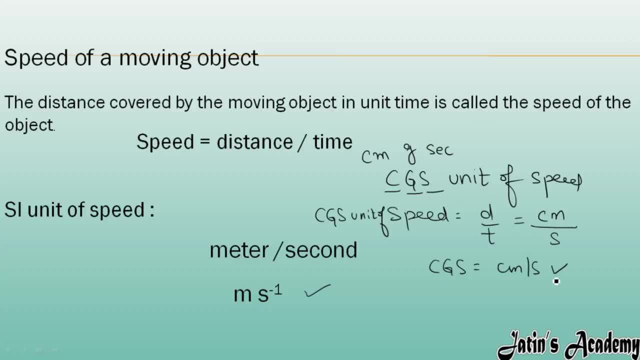 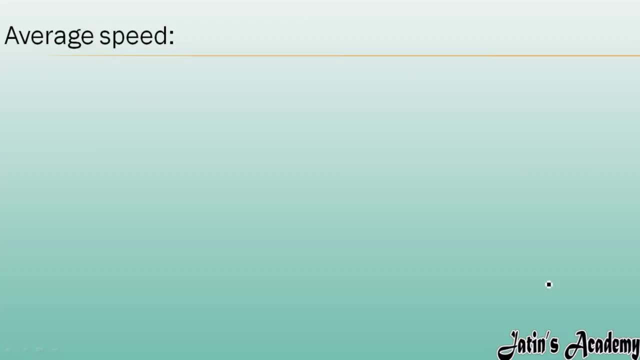 What is the SI unit, meter per second? What is the CGS unit, centimeter per second? fine, So this we have already done. next, We are going to start with the next topic, that is average speed. So what do you mean by average speed? 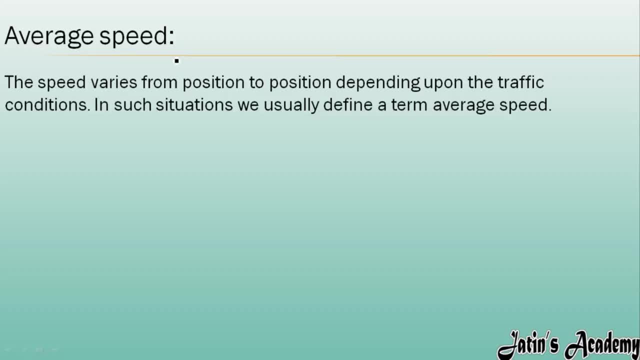 Actually, whenever we are riding our Activa, we are on our car, the speed is not same or we are not covering same distance in same time. Why? due to, might be some traffic conditions, We are not able to cover same distance. So sometimes speed is going to vary. varies means changing from speed is going to change from position to position depending upon traffic conditions. 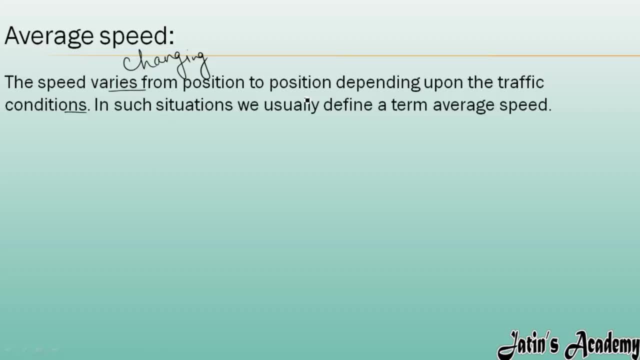 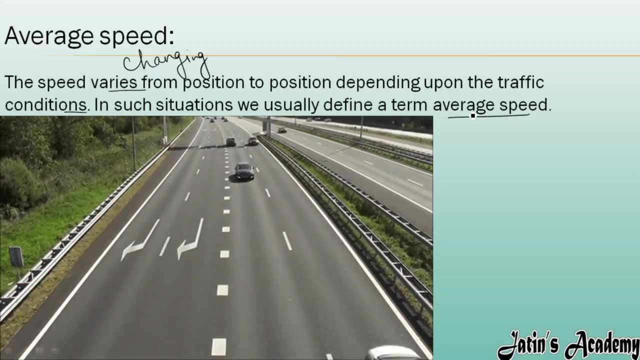 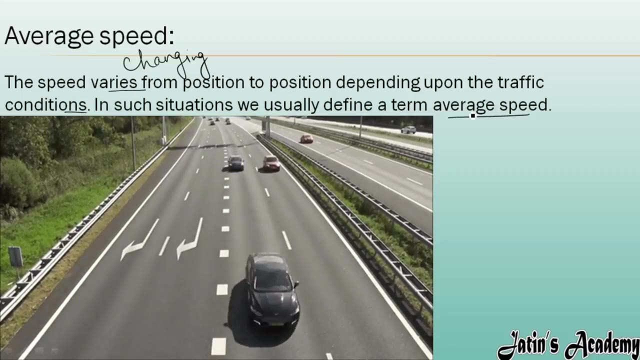 So in this situation, we are not going to see the speed. in this situation, We are going to see the average speed. fine, So here for example, see, due to this traffic and all this, these all cars are not Having their same speed, So their speed is varying from position to position. that is known as its average speed. 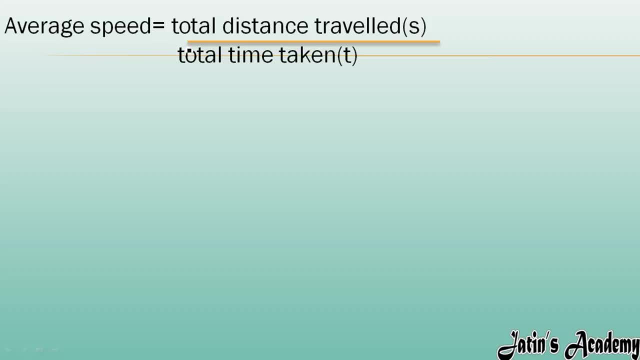 Now see the formula for average speed. as we have learned for the speed, speed is equals to distance. upon time, Now, we will see the formula for average speed. average speed is equals to total distance traveled over total time taken, For example. firstly, this car is here. 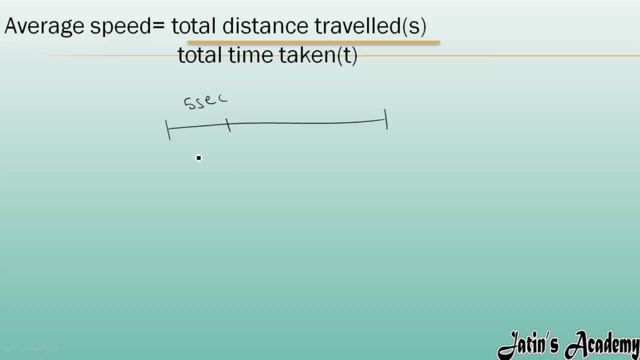 It took, for example, 5 seconds For 10 meter. then it took again 5 second, for example, 25 meter, due to no traffic condition. It going to cover more distance. So accordingly, we are to see the different changing of the distance and different time taken. 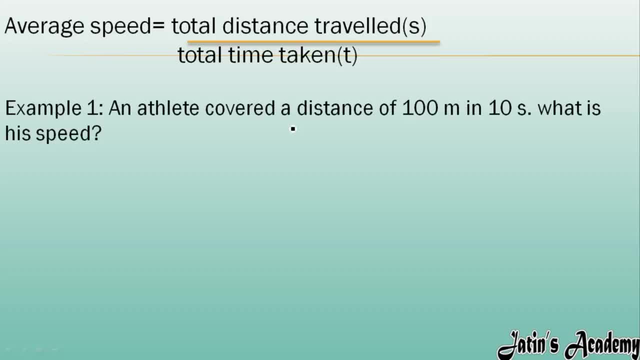 Okay, so we will do one numerical also related to this. So example first: we are having an athlete covered a distance of 100 meter in 10 seconds. So athlete cover distance of 100 meter. So here we are given with distance, distance. 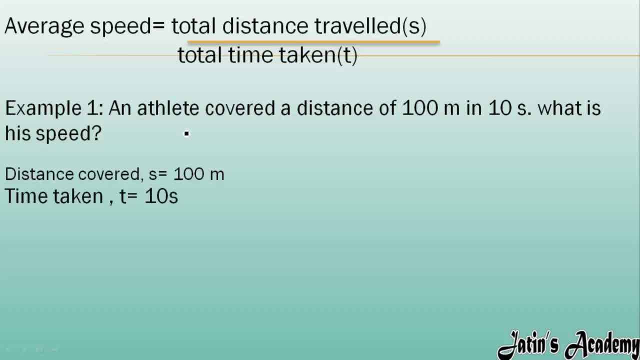 We have given 100 meter, time given is time taken is given, that is, 10 seconds. So, simply, we have to calculate the speed. So might be, as you are, knowing what is the formula for speed. speed formula is: speed is equals to distance over time, distance traveled over total time taken. 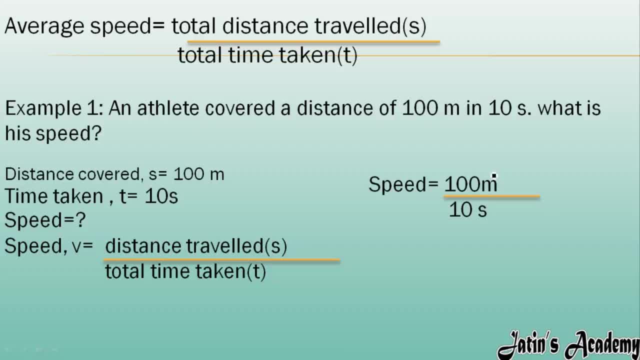 So what do you mean by distance over time? distance is given to us 100 meter. What is the time given? 10 seconds. So simply solve it. It will give you 10 meter per second. This is 0. you can cut with the 0, so it is 10 meter per second as a speed. 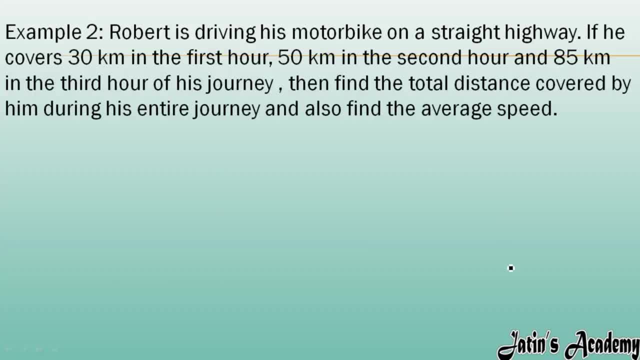 Next we are having: Robert is driving his motorbike on a straight highway. So when Robert name is there, one boy is there who is driving his motorbike on a straight highway if he covers 30 kilometer in first hour. So what do you mean by give what is given to us? 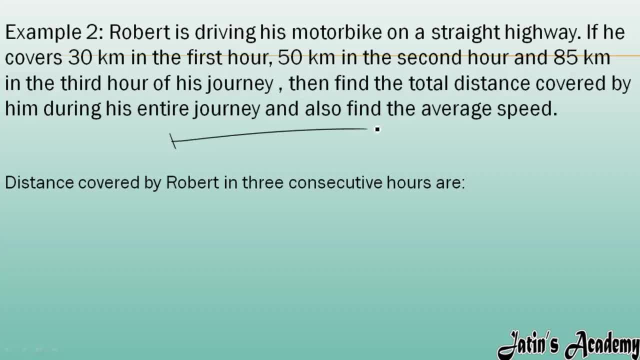 First 30 kilometer, for example, just straight road. in first hour He is covering 30 kilometer, Then in the second hour again in one hour He is covering 50 kilometer, then again in one hour. in third hour He is covering 85 kilometer. actually is given to us. 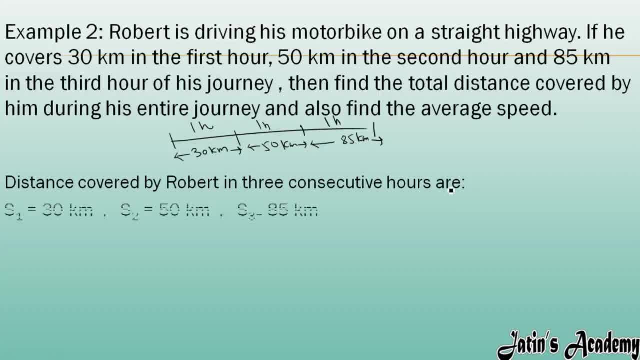 So distance covered by Robert in three consecutive hours are: first distance is given 30 kilometer. Second distance is given 50. third is given 85. So we will firstly find the total distance covered. So total distance covered is plus all these three distance. 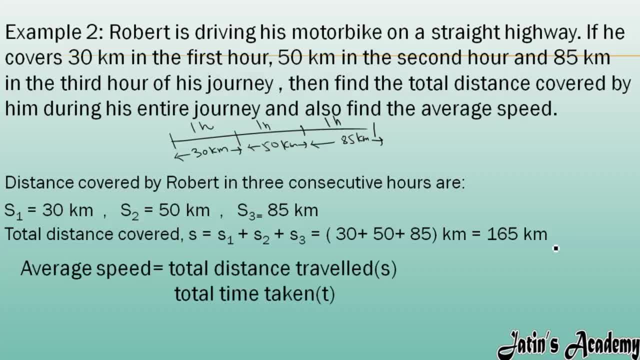 It will give you 165 kilometer. then afterwards we have to see the formula. So formula of average speed is total distance over total time. So what is the total distance? total distance is 165 kilometer over total time taken. total time taken is what? 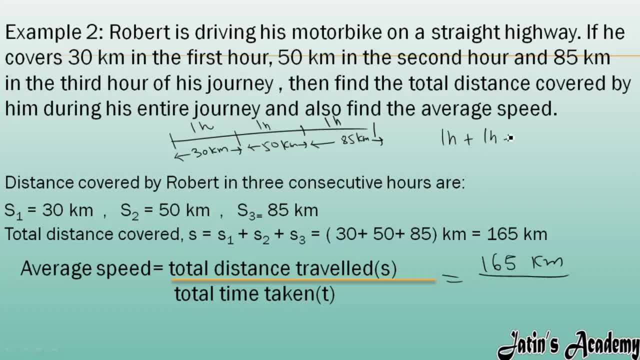 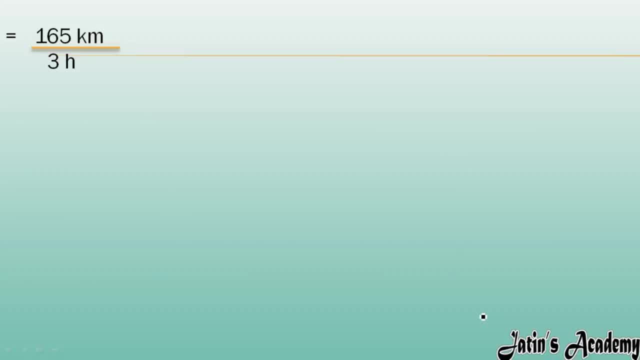 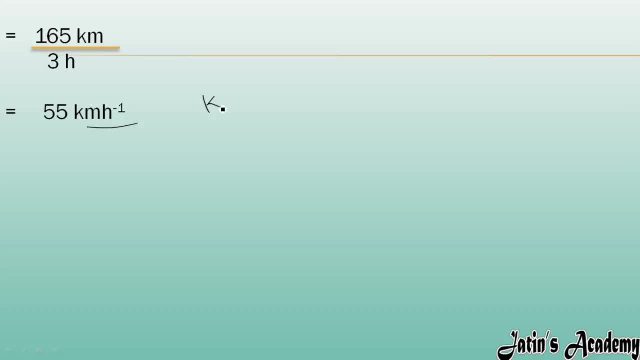 This is a speed covered by a robot. Now see this: kilometer per hour. kilometer per hour is also a unit of speed, but kilometer per hour Is the bigger unit for speed. kilometer per hour is the bigger unit of speed and meter per second is the SI unit of speed. fine, 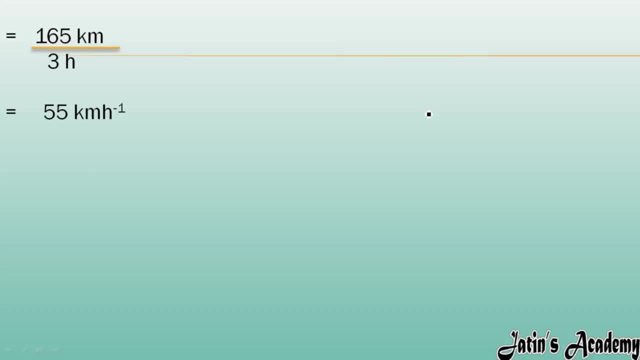 So like this you can solve the numericals related to average speed or related to speed. Next topic we are having here: weight of an object. So what do you mean by weight of an object? The weight of an object is the force with which Earth attracts it. 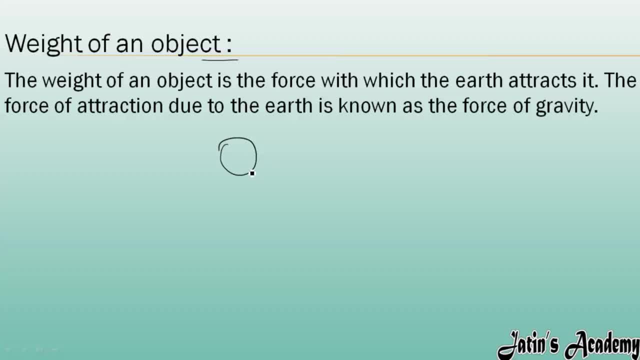 For example, here I am having one ball. when I will throw this ball? Okay, when I will throw this ball? from height. So where this ball will go? obviously it will go down side or it will move upward. No, when we will throw the ball, this ball will move down side. 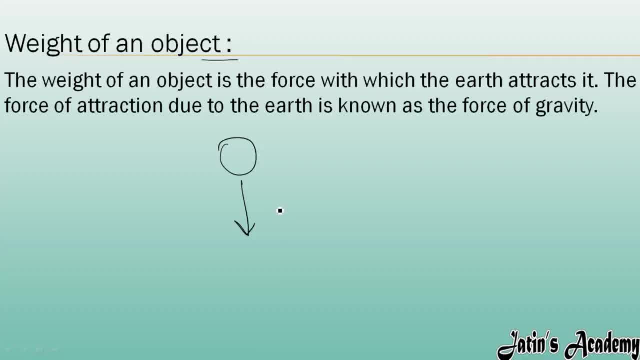 So each and everything? we are knowing that each and everything is going towards the center of the Earth, or each and everything is attracting towards the Earth. by which force it is attracting toward the Earth? This is force of gravitation or gravitational force. in a same way, in a similar manner, each and everybody, when attracted toward the surface of Earth, that force is nothing but is a weight of an object, means the force by which this object is attracting towards the Earth, that force is nothing but a weight of an object. 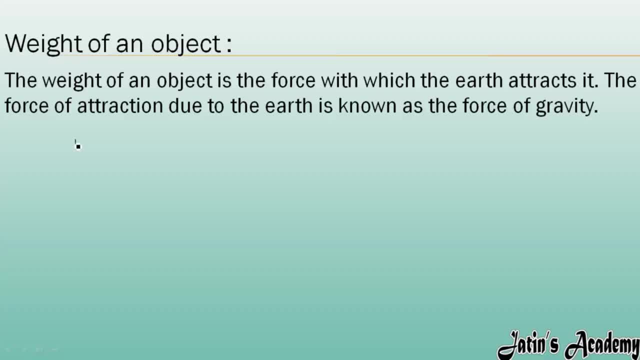 So might be. what is weight? it is clear to you. You can see here mass also. What do you mean by mass? side by side, I will tell you what do you mean by weight. afterwards, We are having one difference between mass and weight. from there, 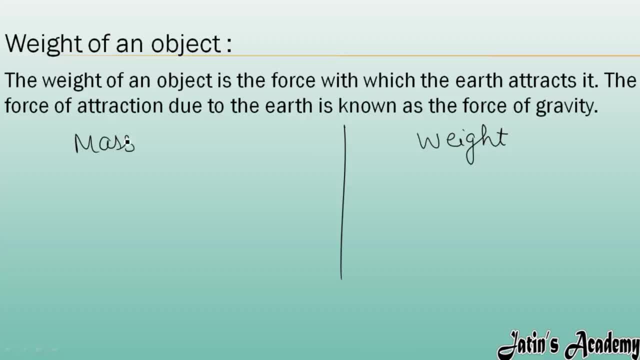 You can note it down, but still here I want to explain you. So what do you mean by mass? mass means quantity of matter contained in a substance. how, for example, this one substance I am having. So in this substance, how much quantity of matter is contained. matter means, as we know, 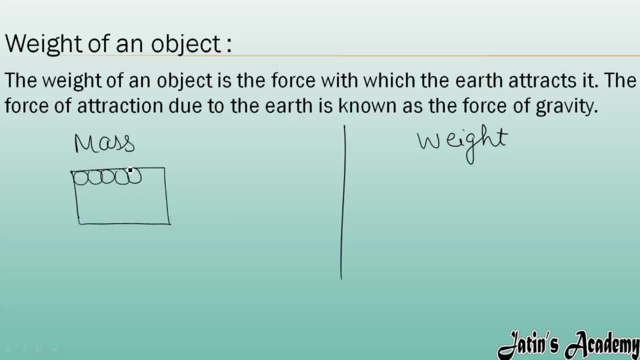 Each and every matter is made up of atoms or molecule, So in this material also, mass is a quantity of matter contained in a substance. in this substance, How much matter is contained? that quantity of matter will give you mass. fine, What do you mean by weight? weight? 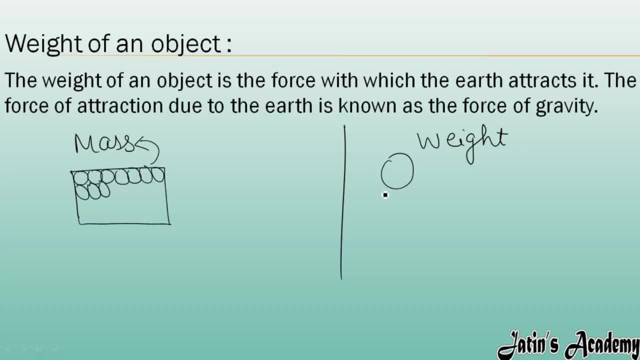 I already told you, each and every object is going to attract towards the surface of Earth with some force, and that force is nothing But a weight of an object. This is the main difference between the mass and weight. Actually, these are the definitions related to mass and weight. 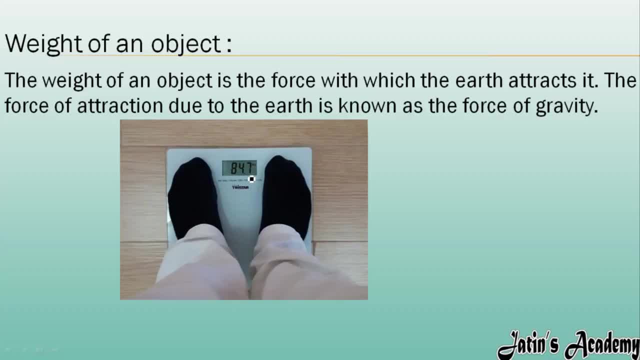 See, this is a weight. when we are measuring, it is giving us the weight next We are having. weight of an object is the force of gravity experienced by an object. This I already told you: whatsoever object is going towards the surface of Earth or falling down, that all objects. 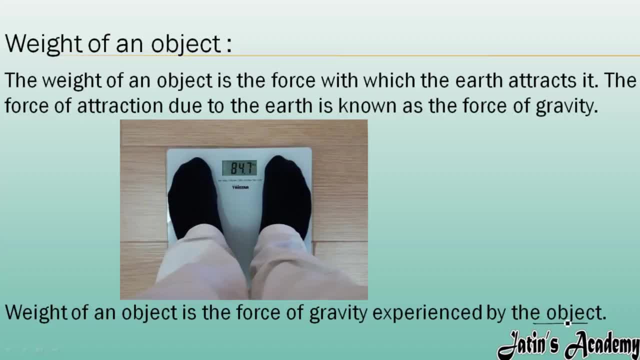 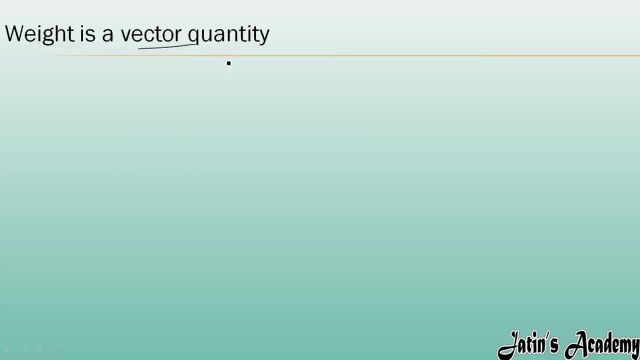 Are having some gravitational force and that force is nothing but a weight of an object. Now we are having weight is a vector quantity. vector quantity, as I already told you, in vector quantity We are going to see magnitude. in vector quantity, We are going to see magnitude as well as we are going to see the direction. 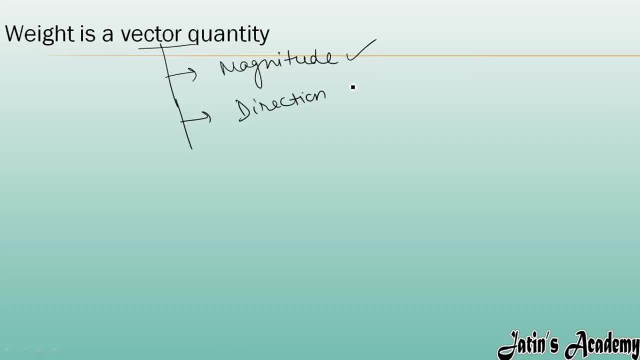 So weight is also a vector quantity in which we will see magnitude and we will see direction. for example, weight is five Newton, so here five. five means magnitude, five is also important direction. Also, weight is applying downside or it is moving upside against the gravity. 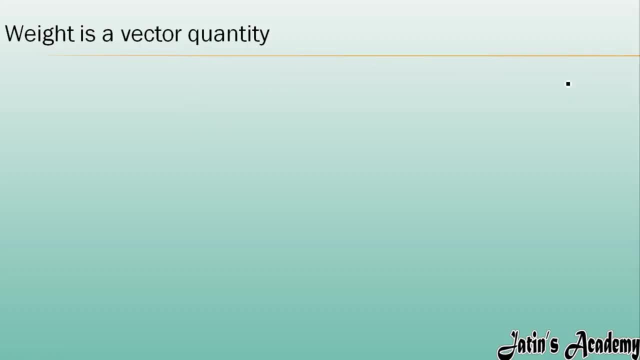 So that is also important. So weight is a vector quantity, but mass is a scalar quantity. in mass We need not any like direction. Why, for example, in this matter, in the substance, these matter particles are there, So these matter particles are arranged in which direction? it is important for you. 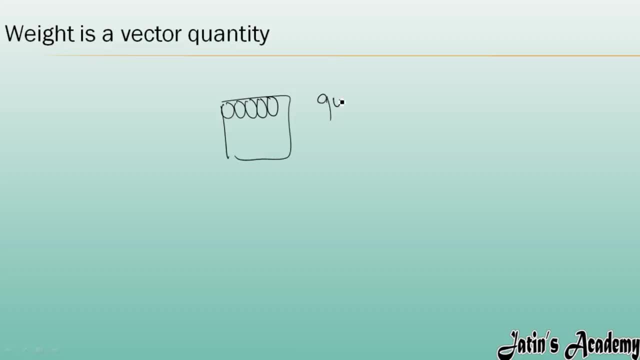 No. so in this only quantity is important, Only magnitude is important. in mass, only magnitude is important, but no direction is important. So mass is a scalar quantity. mass is a scalar quantity and weight is a vector quantity. fine, If M is a mass of an object, G is acceleration due to gravity. 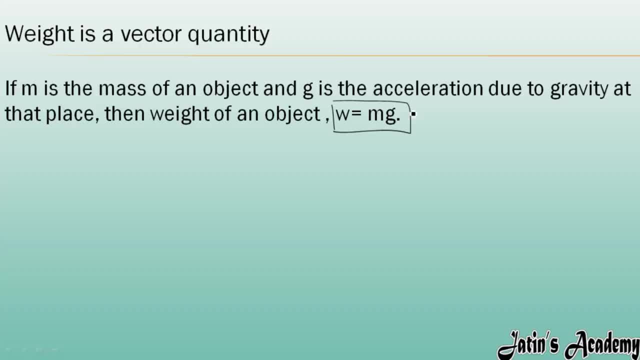 Now we are going to do the relation between Mass and weight. This is a relation between mass and weight. weight of an object is equals to mass multiply gravitational force, That is G, and this G value, this gravitational force of gravity value, is always constant. 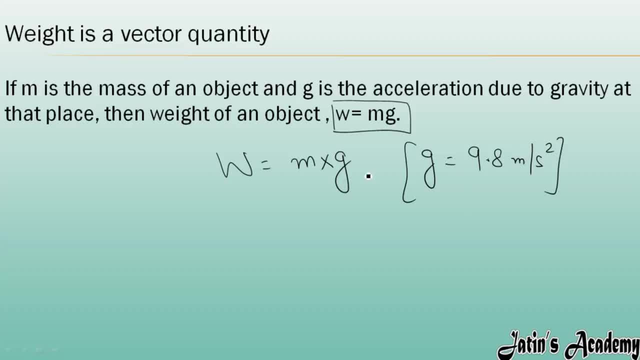 That is nine point eight meter per second square. This value is always constant, This only value we have to put, or in some time books It is given 10 meter per second, also meter per second square also. So this also we can take, but actually it is nine. 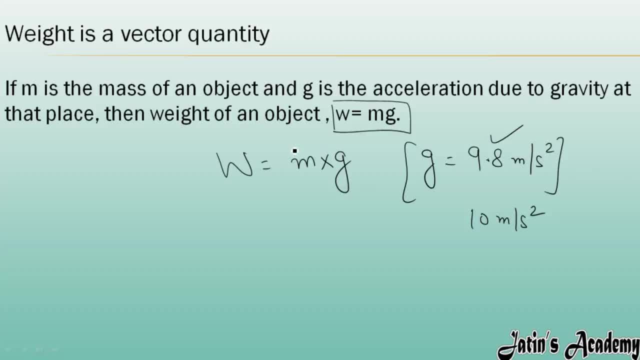 Point eight. So this is a relation between weight and mass, As the value of G varies from place to place. actually, The value of G gravity changes from place to place, as I told. nine point eight meter per second square. This is a value of G on the surface of Earth. 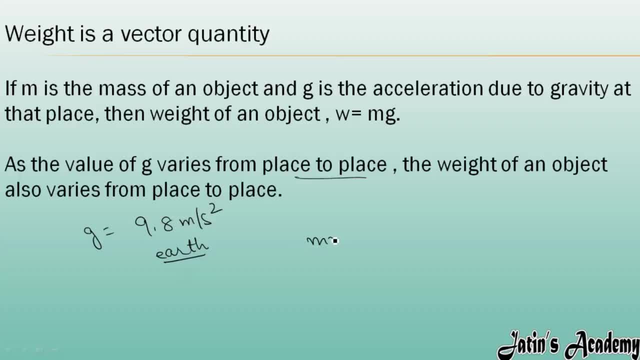 This is the value of G on the surface of Earth. But when we will go on the surface of Moon, Their value of gravity is different. their gravity is less na, so their gravity is different. So gravity changes from place to place. as gravity changes from place to place, 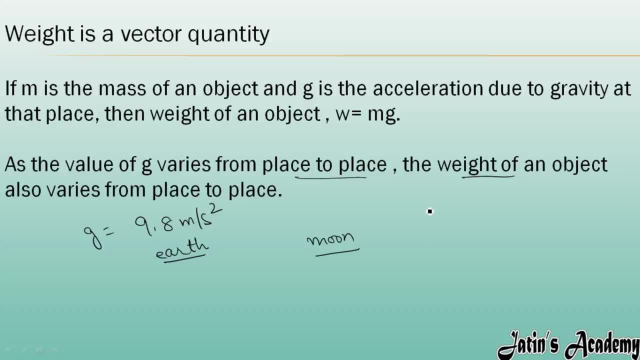 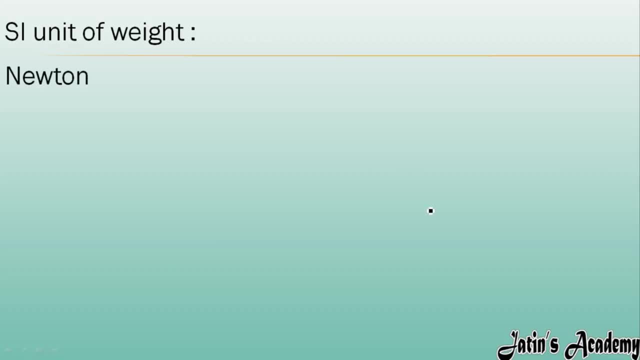 So weight of an object also changes from place to place. fine, Next we are having SI unit of weight. So SI unit of weight is what? SI unit of weight is Newton. Other units of weight which we are going to commonly use, So other units of weight, are kilogram force. 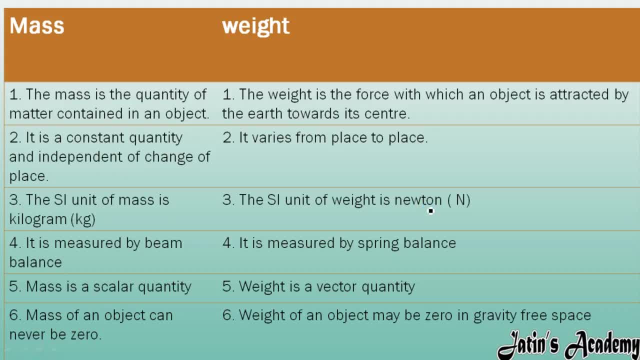 Next we are having kilogram weight. So this is the main difference between mass and weight. First difference is mass is the quantity of matter contained in a substance. Mass means what mass is a quantity of matter contained in a substance? What do you mean by weight? 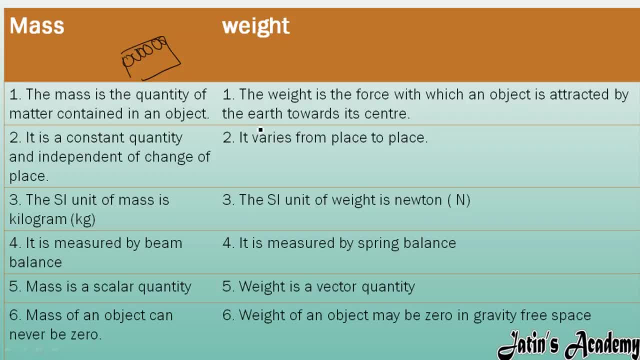 Weight is a force with which an object is attracted toward its center of Earth. when object is attracting, That is known as that force is known as weight. Mass is a constant quantity and independent of place. Mass is a constant means. mass is not going to change from place to place. 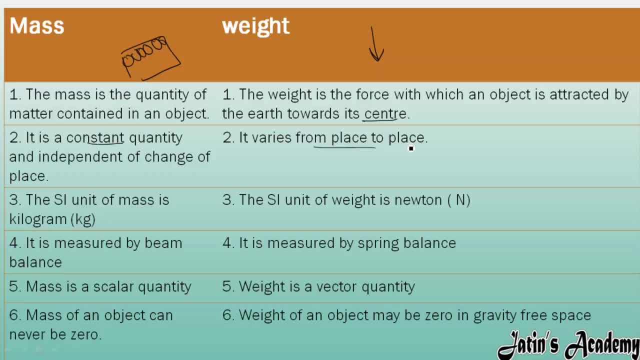 Okay, but weight can vary from place to place. weight We can change. for example, on the surface of Earth weight is different and on the surface of Moon, due to change in the value of G or gravity, The weight is going to change. SI unit of mass is kilogram. 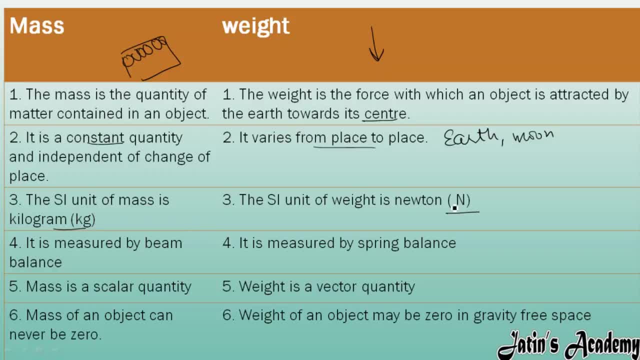 SI unit of mass is kilogram and SI unit of weight is Newton. Actually, weight is what? weight is a force only, and force SI unit is Newton. Similarly, weight SI unit is also Newton. Mass is measured by beam balance. Beam balance might be. you have seen this kind of thing like this: two pans are there. 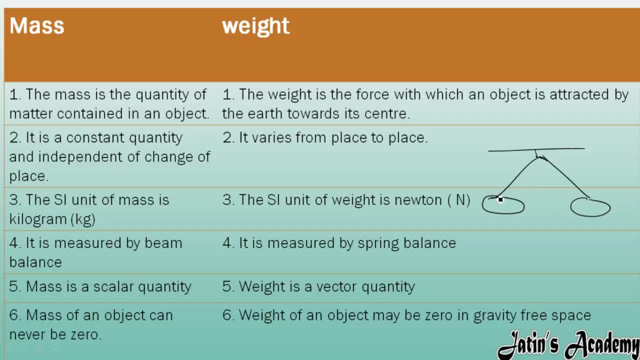 Here. string is there. These two strings are there. This is a beam balance, and weight is measured by space- Spring balance. in the next slide I'm going to show you spring balance also. So mass is a scalar quantity which is only depending upon magnitude. 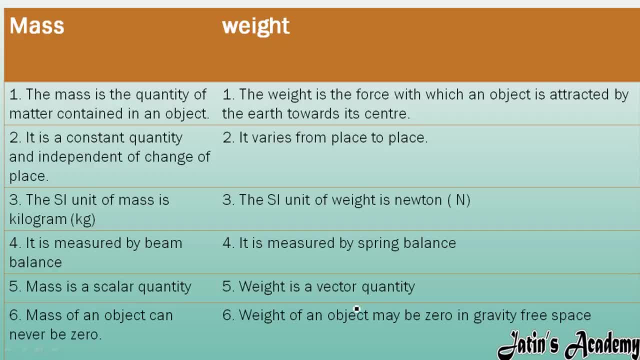 but no direction is important. Weight is a vector quantity in which both magnitude as well as direction is important. Mass of an object can never be zero. mass can never be zero Why? because in matter some quantity of matter should be there. no, in any substance. 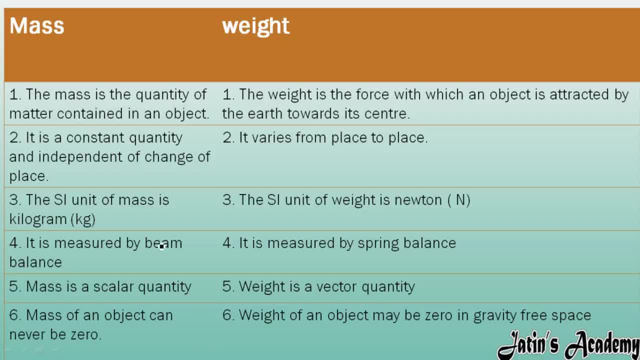 Any quantity of matter is always there. So mass of an object can never be zero. but weight of an object can be zero where it can be zero in a gravity-free space. gravity where there is no gravity, where there is zero gravity. So in that places weight can be zero. 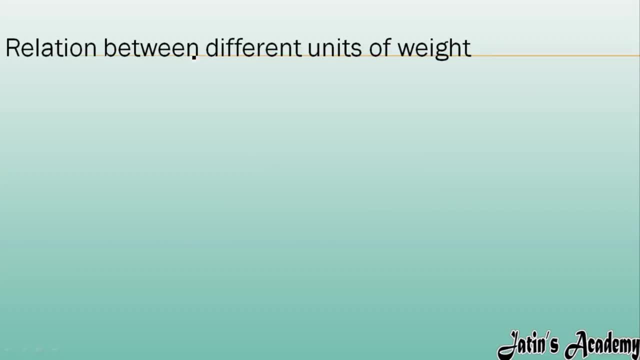 Okay. So next we are having relation between different units of weight. as we have learned SI unit of weight, that is Newton. afterwards We have learned kilogram force or kilogram weight. So now we are going to see the relation between different units of weight. 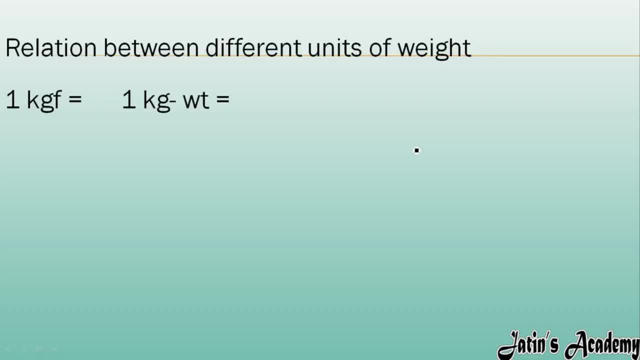 So first is we are having relation between kilogram force and kilogram weight. One kilogram force is equals to one kilogram weight means kilogram force and kilogram weight. They both are same, only kilogram kilogram, same only here. force is nothing but a weight only. 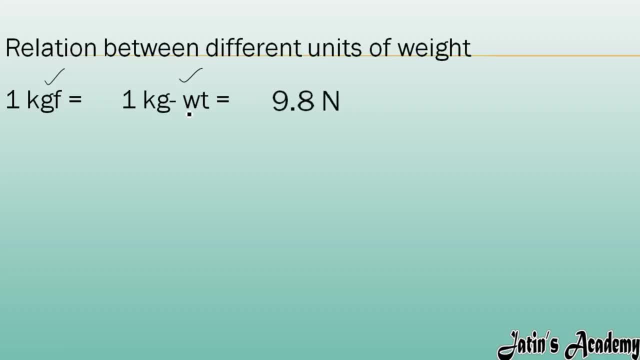 So one kilogram force is equals to one kilogram weight and they both equals to nine point Eight Newton. It is very important from exam point of view. They can ask like this: like one kilogram force is equals to dash Newton, So in dash how many Newton, nine point eight Newton. or they can ask one kilogram weight. 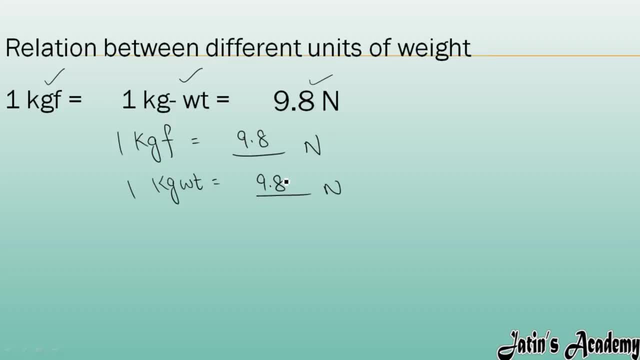 equals to dash Newton. That is nine. point eight, Newton is the relation between kilogram force and Newton. plus it is a relation between kilogram weight and Newton. next, we are having some multiple of kilogram forces, gram force, if we will see the sub multiple or the smaller unit for 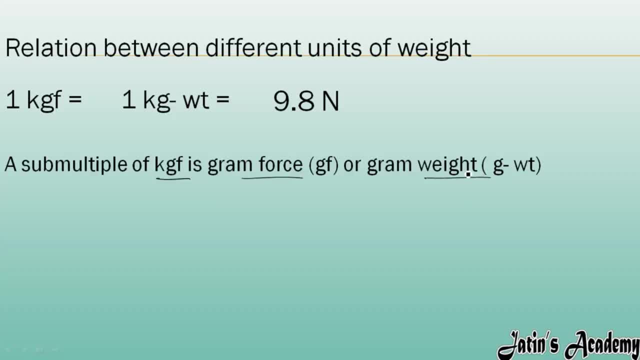 the weight, that is gram force or gram weight. So some multiples of weight are gram force and gram weight. So relation is: one kilogram force is equals to one kilogram. for one gram force is equals to one gram weight. gram gram- same force is nothing but a weight. 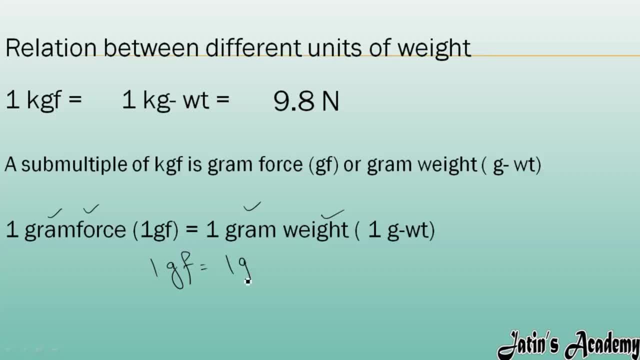 So one kilogram, One gram Force is equals to one kilogram. So one gram weight, fine, One gram force is equals to one by thousand kilogram force. here how it came here. actually, one gram force is there in one gram, as we know how many kilogram are there in one gram. 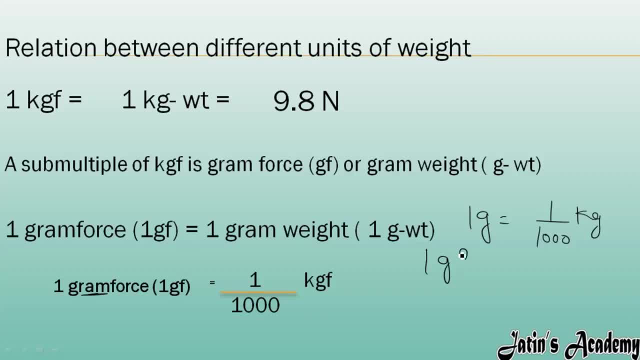 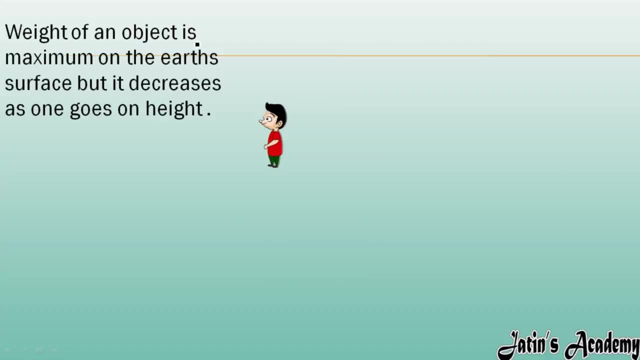 one by thousand grams are there. So one gram force is equals to one by thousand kilogram force is same. So this is the relation between kilogram force and gram force. fine. Next we are having weight of an object is maximum on Earth's surface, but decreases as 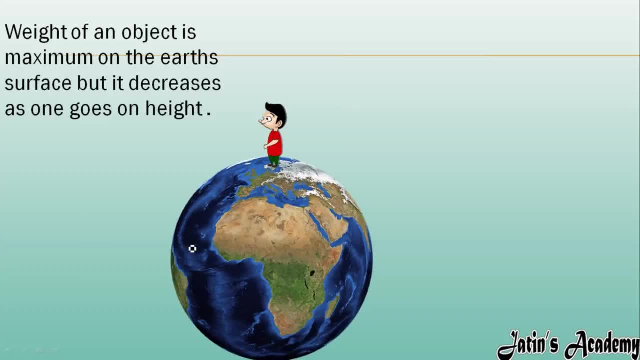 one goes on height, for example. this is the Earth's surface, the Earth, when we talk about the Earth's surface surface, means this full part in between the Earth, this full part. in this full part, weight is maximum, weight is there, But as an object Is going on some height. 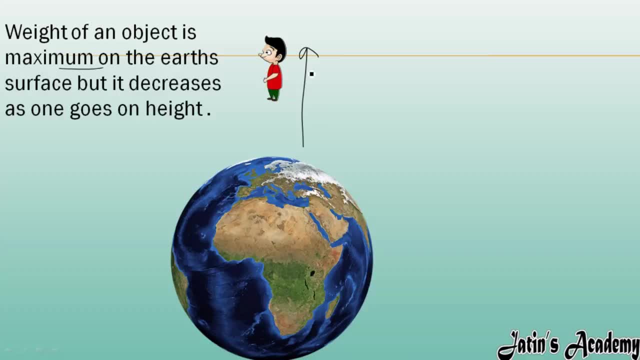 This object is going on some height. when any object is going on some height, at that case weight is going to decrease. at that this case weight is going to decrease. but when object is there on the moon surface, their object weight is maximum. On Earth's surface, weight is maximum at its poles. 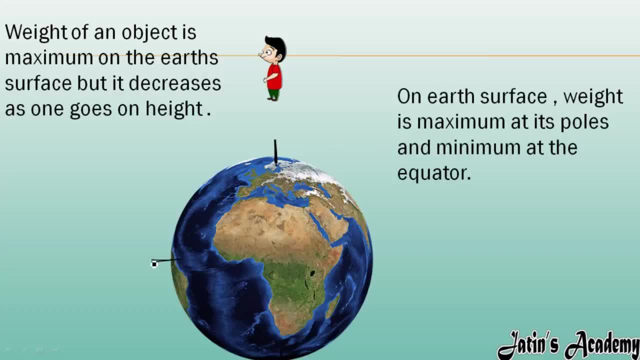 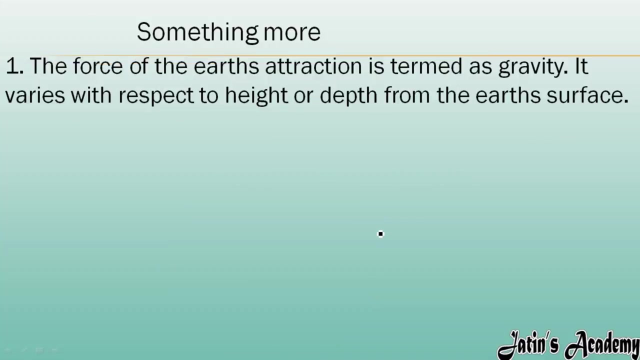 Poles means this one, this is also pole, This is also pole, Here also pole. Four poles are there. ok, So gravity weight is maximum at the poles and minimum at the equator. This is equator, central line. So at the equator weight is minimum and at the poles, great weight is maximum. fine, 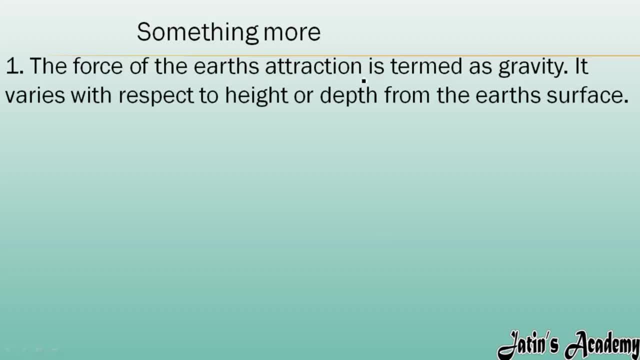 Now we are having some more knowledge. The force of the Earth's attraction is termed as gravity. this we have already learned: that whatever force By which object is going towards the Earth, that force is nothing but a gravity. and this gravity varies from height to height or depth to depth. fine, as I already told when we will. 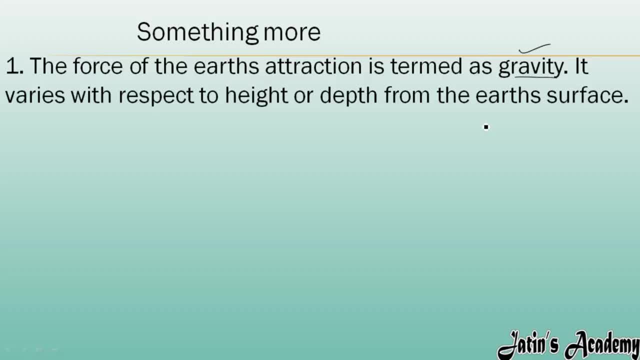 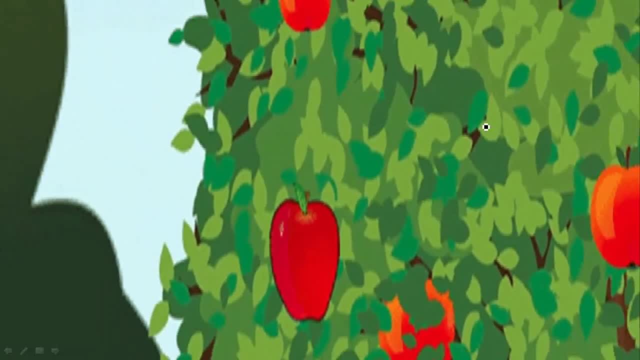 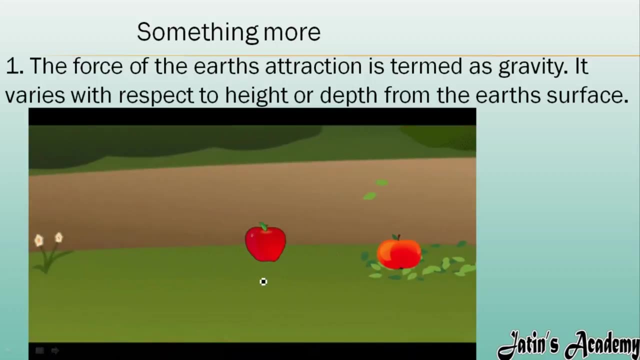 go up the height. when we will go above the surface of Earth their weight decreases, but on the surface weight will be maximum. So next we are having like this: each and every object is going towards the surface of Earth. So this object is also going towards the surface of Earth and at some height it is moving. 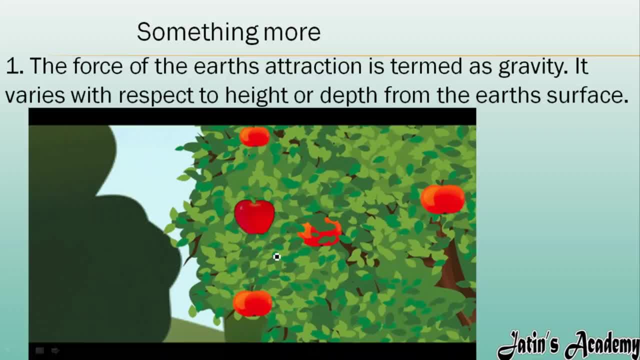 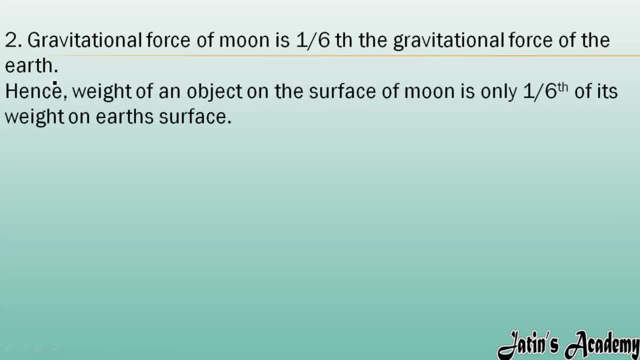 down side due to the gravity or the weight is there. Next we are having gravitational force on Moon is one by sixth of gravitational force on Earth. What does it means, for example, on Earth? on Earth, my weight is 60 Newton. on Earth's surface, my weight is 60 Newton. 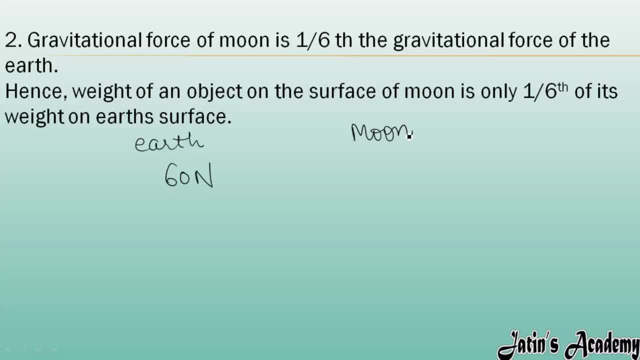 But when I will go on Moon's surface, I will go on Moon's surface, I will go on Moon's surface. There it will be one by sixth, only one by six of weight of Earth. If I am having here on Earth 60 Newton force and I will go on the surface of Moon, then 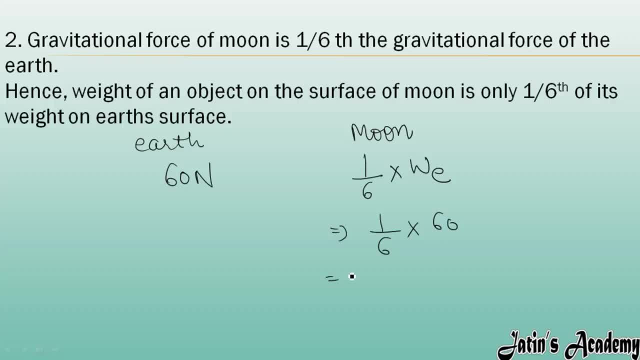 my weight will decreases. to see here 60 value. put here 6, tens are 60. So there, my weight is only 10 Newton. So what does it means? gravitational force on Moon is one by sixth of gravitational force On Earth. fine, So if you want to calculate here, it will be like this. you can write: sorry, gravitational.